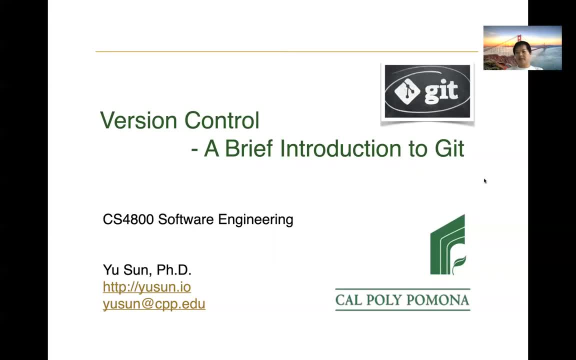 at that time I asked students how many of you have have used Git. Probably one fourth of the class raised their hand, Which was very impressive. And today I asked you how many of you have done Git? Probably I would say 80%, 90%, probably already are doing that, So I don't need to spend too much time. 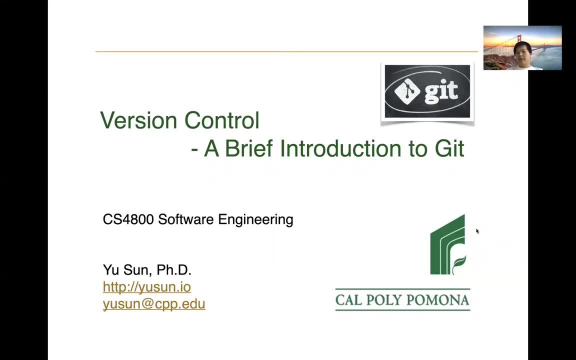 talking about this one. However, there are still some of you who have not used Git before, or you don't even know what Git is, or you don't even know what version control is, And then you really need to pay attention to this one And then, after the class, try to use. 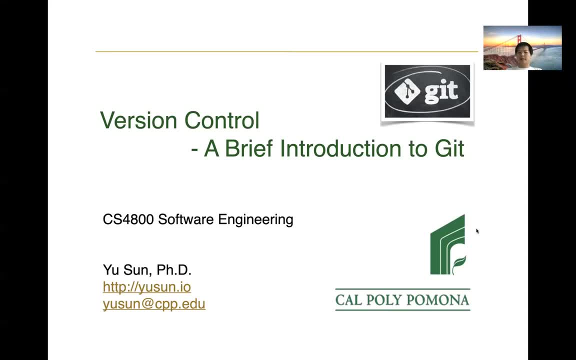 Git and start to use that Heavily. All right, This is a very fundamental skill for you to work on software. All right And all right. so let's actually look at the version control. Okay, so why do we ever need? 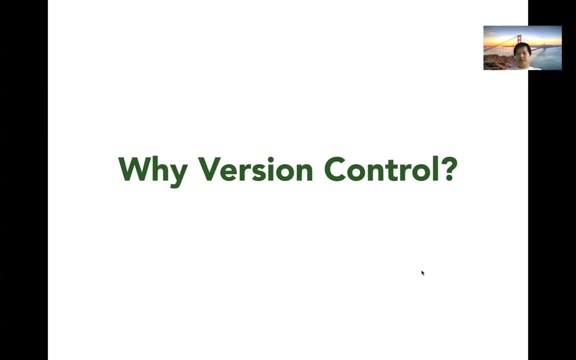 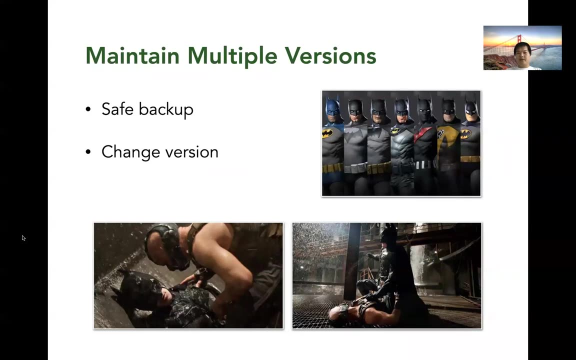 a version control. What is version control? Pretty easy to understand: you're trying to control and manage all the versions of our software, right? Think about different reasons. All right, Initially I'm sure a lot of you have had this kind of experience. we want 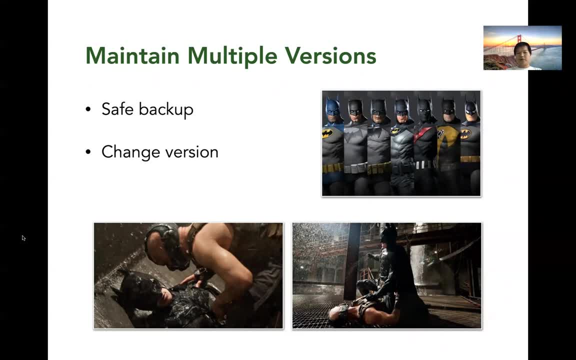 to just have some kind of backup for your- you know- software. Let's say that you wrote some software or some code in Eclipse or IntelliJ right And make a lot of. you have some kind of experience that you work on a very complicated course project that takes many days to finish. 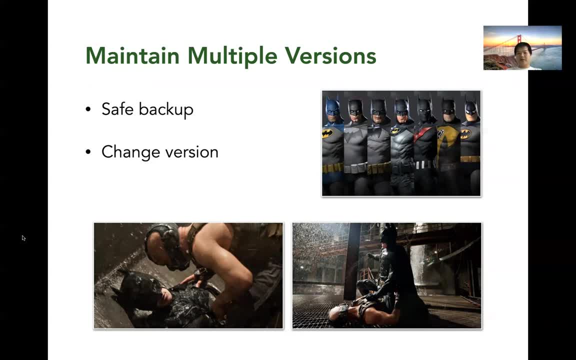 Eventually, you fix all the bugs, you got a really nice version. you feel you've done a lot of work, and then you don't want to lose your work, right? One thing we can do is to open the folder with the file- and I would just make a zip file- And to save all the 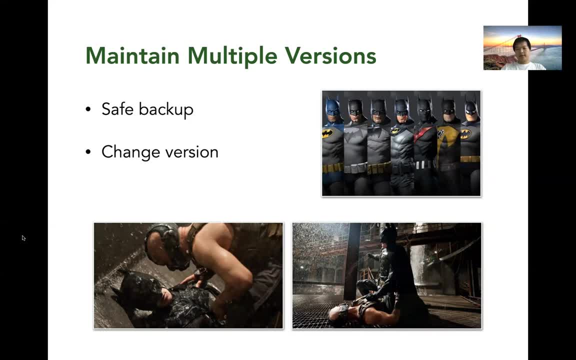 version I have so far because I know this is a working version, And after that I will probably also email that zip file to myself, Because I know in an email it will be kept in the email server, not my disk. So one day if my computer died and I will lose all my 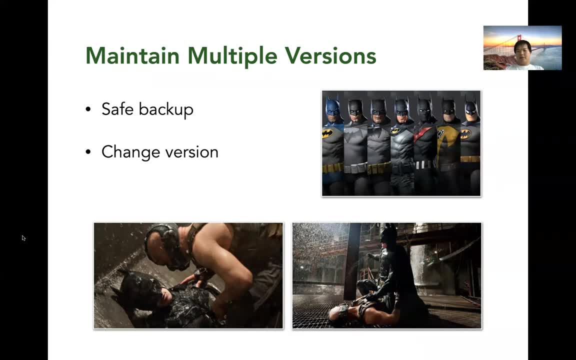 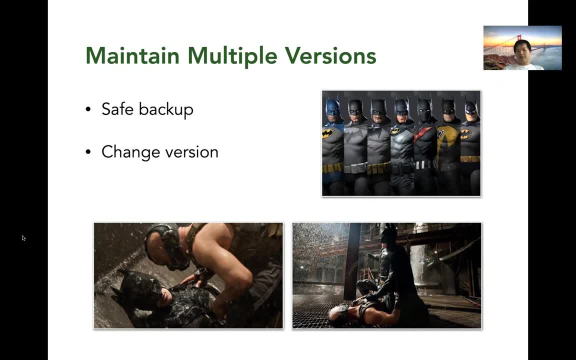 All right, And of course today we will use Google Drive or some other. you know color drive And but that's why we're trying to. you know what's the motivation about using some of the version control tools? because we want kind of a backup. something happen. 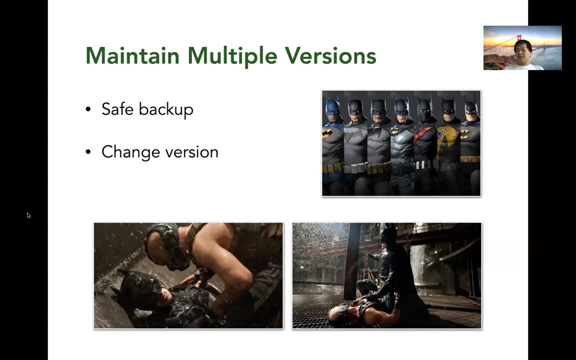 I can still roll back. And also, there are every software versions, even though your software are all correct. but for some reason you do want to change the different versions. maybe a computer, the OS, is too old, then you cannot support the newer version. I have to switch that for some other purposes. 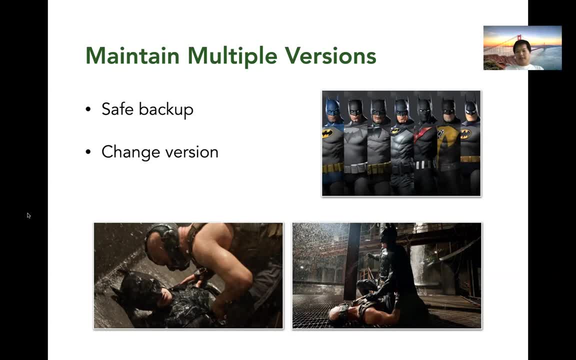 And in software development world you often need to rely on the dependencies. Sometimes the version doesn't matter. sometimes the version matters a lot. So you need to specify the version. you need to change the version, So we need to have two to help us manage a different. 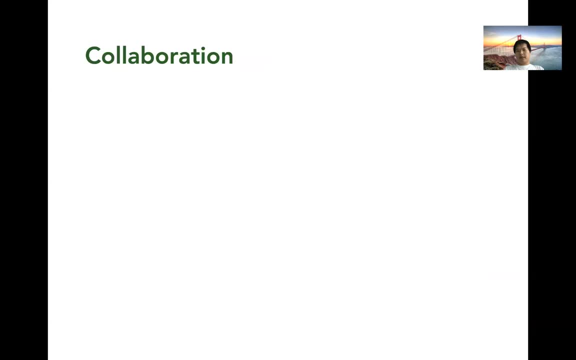 version. Another one is about the collaboration. So when you work with a software team and you're not just yourself writing a code, multiple developers work on the same code base together, and that's going to cause a lot of collaboration issues. So let's. 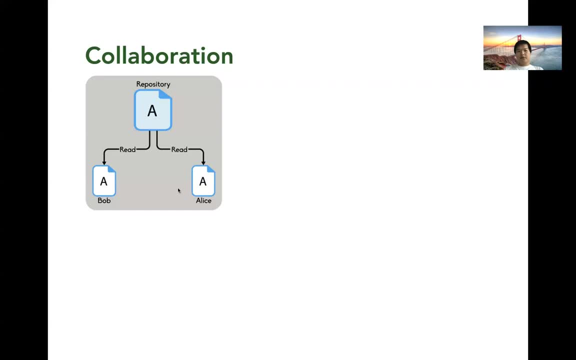 take a look at some of these scenarios. This one pretty much explains how the version kernel works. why do we need that? So let's assume that there are two developers, Bob and Alex. They're both working on this software repository, the code base here. 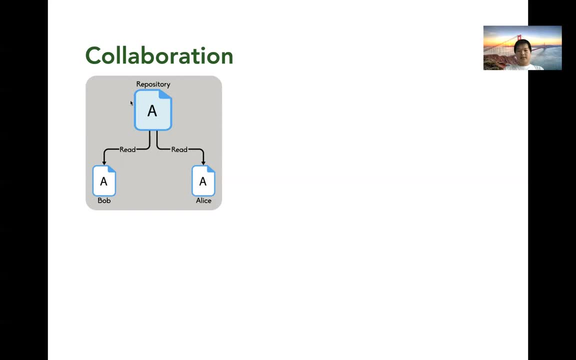 And then let's say this: this is a centralized copy of the code base. And then both of them started working on this in parallel because they're the same team, So they both read and get a copy of the software. And then they started to make some changes. 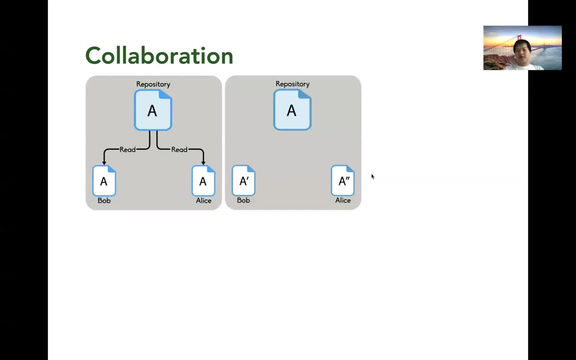 Bob make one change, one feature, and then Alice makes a different feature. After that Bob pushed his code back to the repository to update the copy because he finished his feature And then, so that time the repository has a different version, updated version. 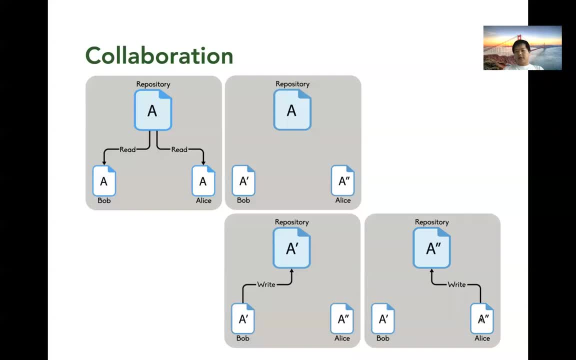 which is the same as Bob's, And then eventually Alice also pushed her changes back to the repository. At that time this repository has another updated version. So did you guys see the problem here If you do this kind of a way to kind of update? 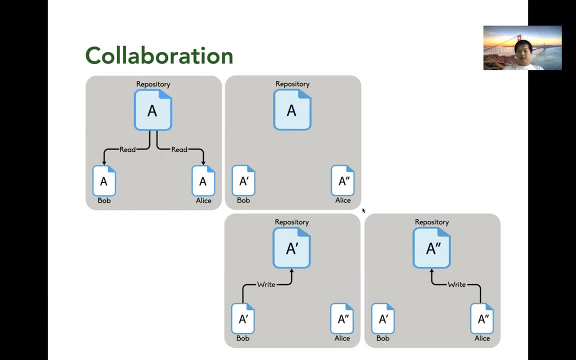 your repository and copy. So yeah, I'm not gonna ask, but obviously this one here. you update the repository, but, Alice, just simply overwrite this copy, which will totally overwrite Bob's change. All right, because this one happens after Bob, all right. 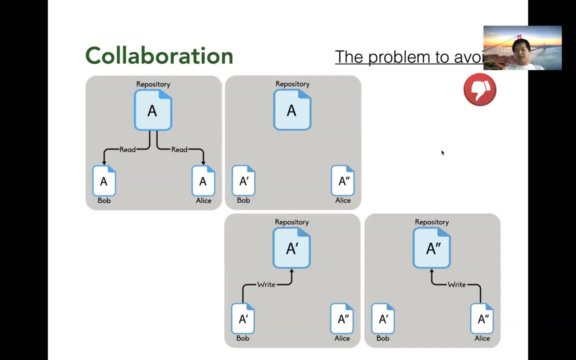 So that's a very bad problem. you wanna see all right, So you work with a team, but then when people are pushing and getting the code back, they are overwriting and trying to change. That's actually very, very bad. So we need to think about how do we avoid this problem. 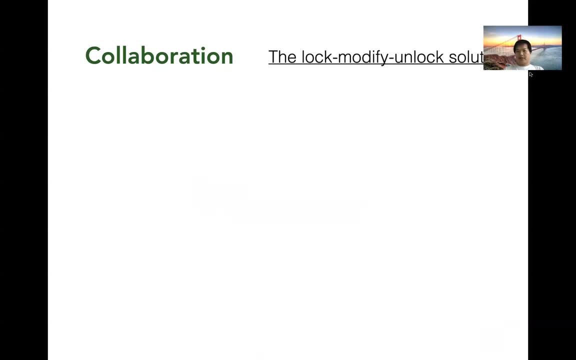 Right. So a lot of the solutions are based on this kind of maximum using some kind of a lock. So for those of you who have done operating system course probably have understand or learned this concept of a lock right. So anytime when you have a resource that had to be shared. 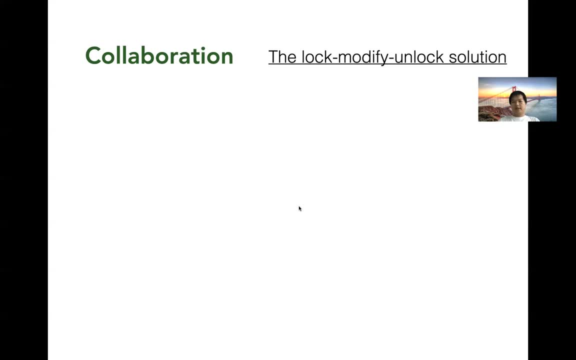 or cannot be shared by multiple parties. then we can always set kind of a locks: Whoever has a lock or has a token can access it. Otherwise people have to wait for the lock. all right, So that's a very typical. so you can do this kind of locking. 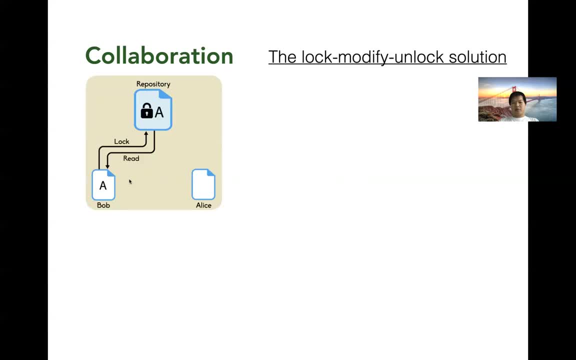 All right. so I have a repository here and Bob has tried to work on it and Bob gets a lock first So he can actually read the copy, And but Alice can't do this because Bob has a lock. The repository has been locked, nobody else can touch it. 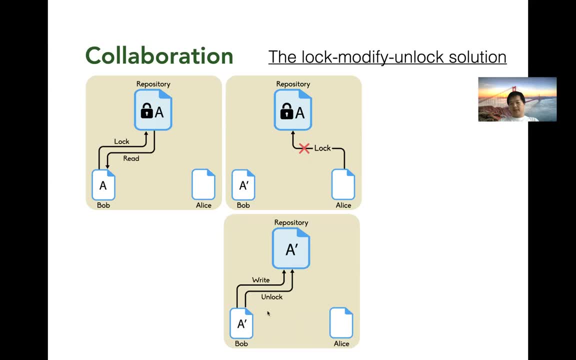 All right at that time and then Bob can be free to read and write everything and update the repository eventually, And after that Alice can grab the lock, after Bob releases the lock, and then get the updated copy right. So in this scenario, 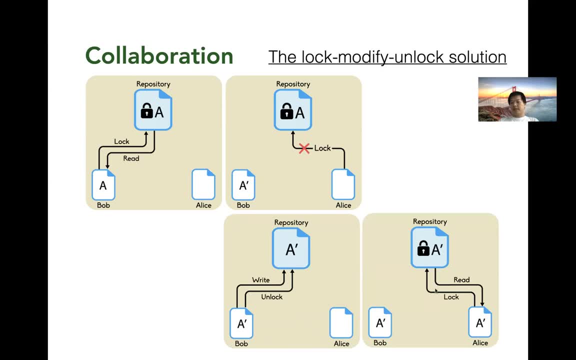 we do not have this kind of override problem, because the moment you are getting a lock, you get the most updated copy, all right, And then you just make your change on top of it and it remains everyone else. change happens before, all right. 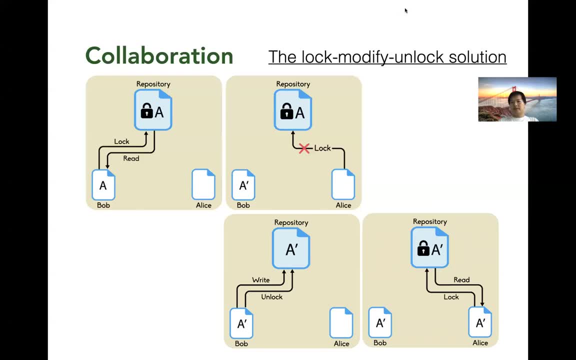 So my question here is: is this an ideal situation? Because what would happen if I did exactly the same thing? or onto a software like I did before? And the worst time is when counsels come and go to the end of theäll. 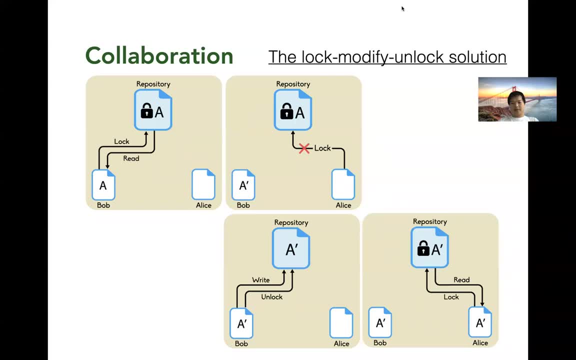 guess I'll give you an example of a large team- Okay Windows team- in Microsoft. They're all based in Seattle in the headquarter. Does anyone know how many people are working on a Windows and for the, for the whole like Windows product? 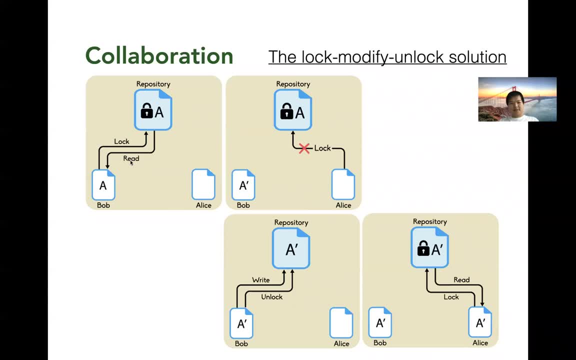 Windows team guys. Give me a guess How many developers are working in a Windows team in Microsoft? 20,000? Sorry, Oh good, Jason, Yeah, it is 5000.. Yeah, 5000.. The number I heard about five years ago. I don't. 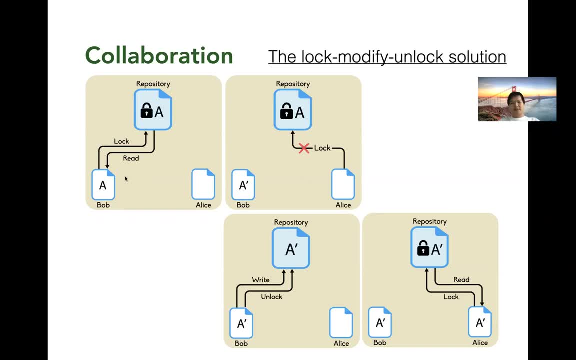 expect to be big changes, because Windows is not going to be the major only product. Microsoft is actually doing pretty good recently on their cloud computing, the Azure platform, So that's definitely their major focus. Windows office is important, but I don't expect the Windows team to be. 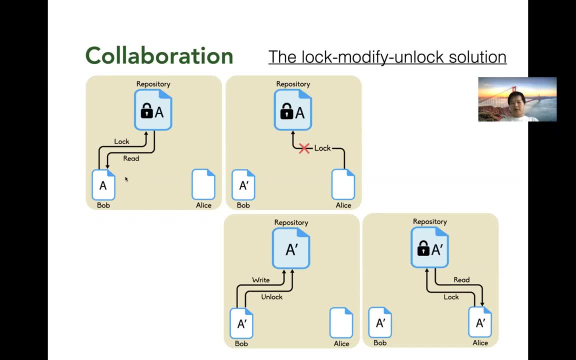 expanded that quickly. So about 5,000 people are in Windows team. I also know the Windows kernel team, the most important- I won't say the most important, but kind of a kernel that's in the lowest level of OS That team has. 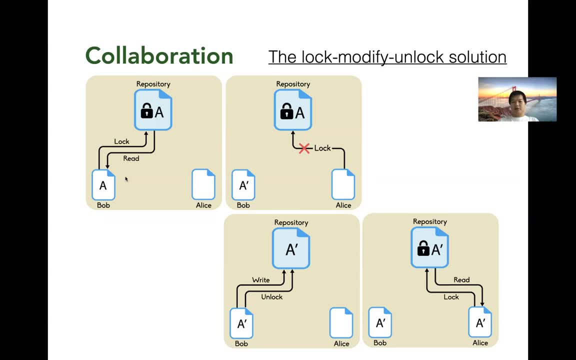 about 30 to 40 people just writing all the C assembly code to do the kernel, All those low-level stuff. But think about when you have a team of 5,000 developers. this approach is not going to work. So the modern approach is: 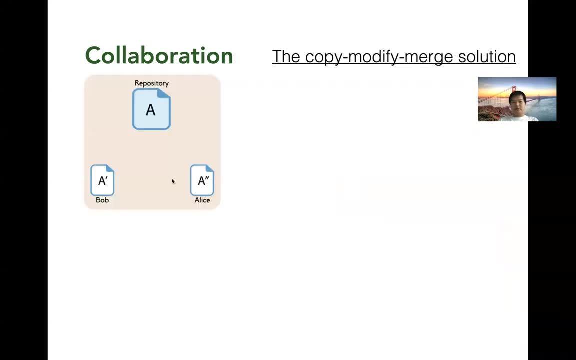 something called a copy-modify-merge solution. So let me go through this very quickly. So we should not prevent people from loading the code, even though there is a chance that they can override it, but they can at least get the copy and then start working on it in parallel, because there's no point. 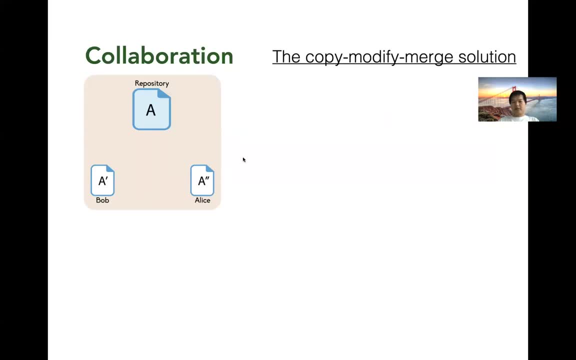 to have people to wait on reading it, So they both get the copy and then they start to make all the changes. Sorry, I think this image is wrong. This should be the second one. All right, But anyway, this time Alice finished her. 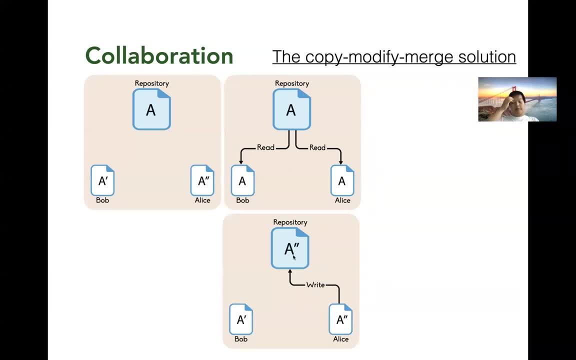 changes first, so she will actually write it back. But in this approach, every time we write a change in the back, we want you to compare your copy with the actual repository copy to make sure your version is based on the current repository version, So they have some kind of version number The moment you. 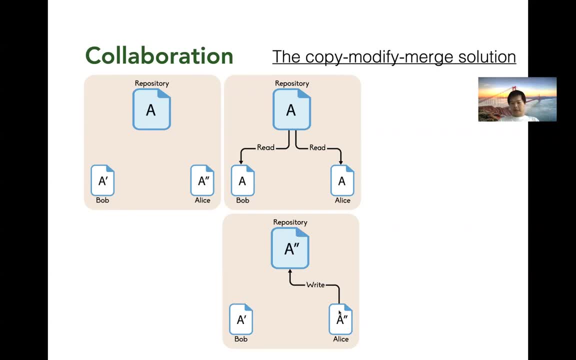 check out the copy. you know the version. you check it out and then, the moment you write it back, we want to see: okay, are your changes based on exactly the same version number? If that's true, then you can write it back, because that means nothing happens after that. So you are free to check it back. 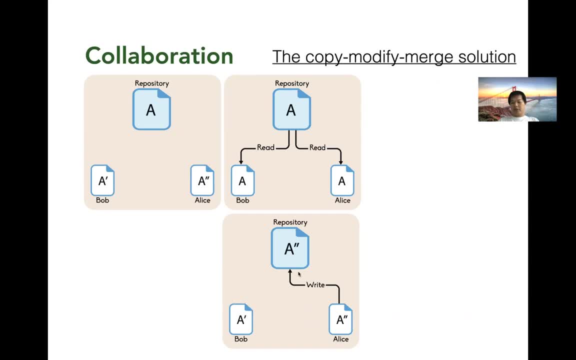 So I'll finish her and she goes back and then Bob at this time also finished his. He is trying to write things back but the the repository rejected because when they compared they got the same version. So we will write it back version they find out the Bob's version is actually older because there's 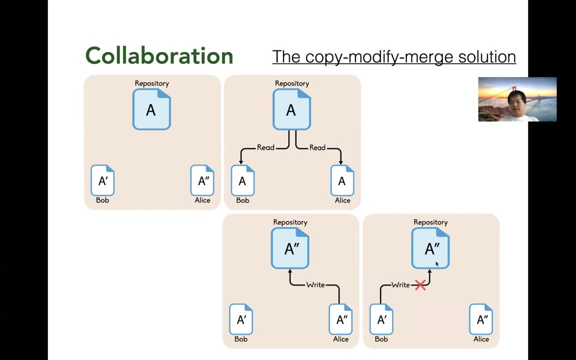 already an update that you don't have all right, so you cannot write this back because that will overwrite other change. so what happened here is Bob need to reload the current code back to his repository, get the latest version, and that time he will need to do some kind of merging. okay, the merging could be. 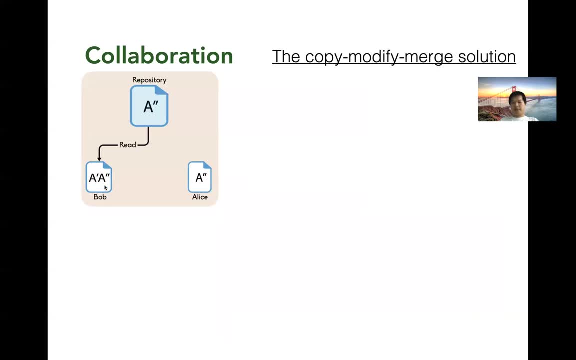 pretty simple, straightforward, because the change are not happening in the same file or it could be a little bit tricky that you need to solve some of the conflicts. all right. after that Bob got another version update the version based on the new code base. at that time, when he try to write the things back to the 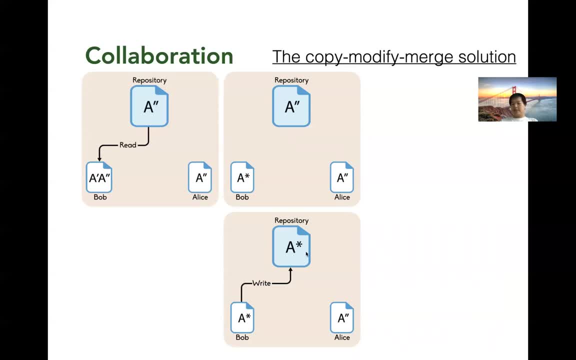 repository. that's allowed because that version is consistent and no other change happened during that time. and after that Alice can also resync the repository, get another updated version. all right, so that's basically how most the version comes out to today. work now not not only get, but also a lot of other tools. I'm not sure if you use. 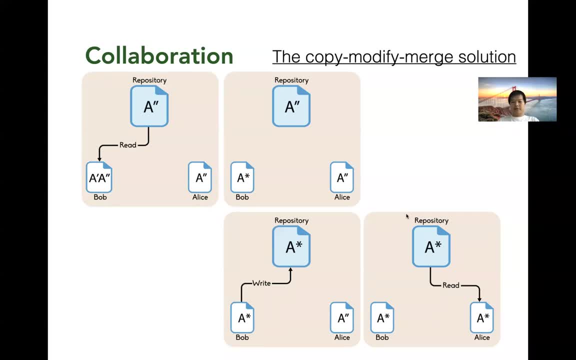 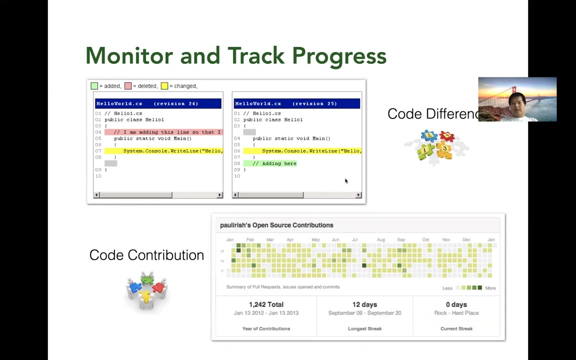 other versionable tools, but get no right now. definitely the most popular, but you know all these are so many other choices, but there's a theory here, almost the same. all right, so that's a recommended approach. and other good things about tracking using the version control: you know it allows you to highlight the 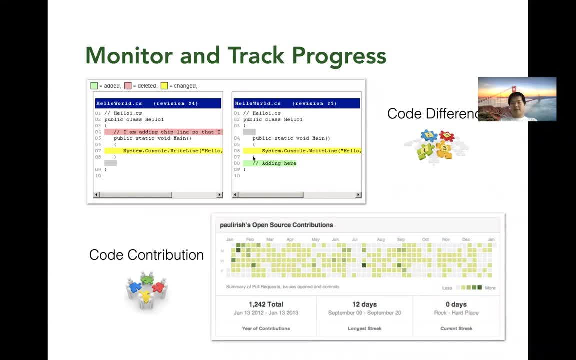 changes easily so you can see what people have done to change the code some. the tool I get, hobbyist, also allows you to figure out some of the contributions your, your community history, alright. so in order get how repository, you can also very easily find out the number of contributions and 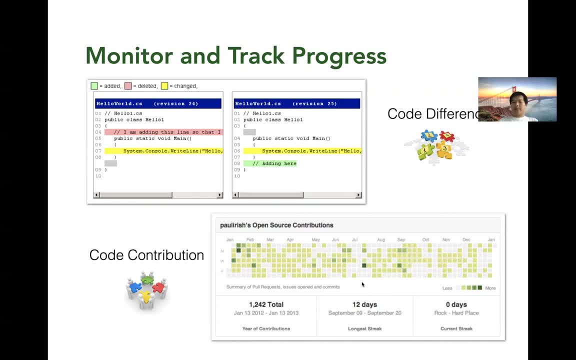 number of changes you are committing to the repository. okay, pay attention to that number. I that I don't mean that number means everything, but that stuff is something we will look into at the end to determine your contribution. because it's very easy, because you've already seen what I got. the other part in the 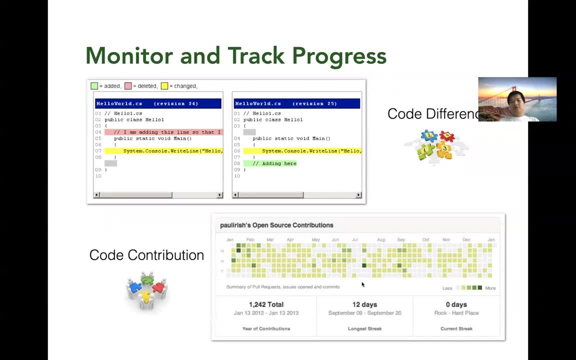 your teammates made 20, 30 commits. you only made one or two. I think there will be some kind of problem. I doubt you will say that you actually helped a lot with your team. And also, guys, do not at the end, okay, never, ever tell anyone, not just me or other instructors. 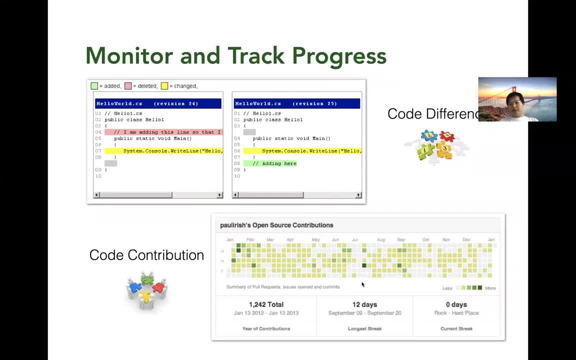 that. oh, you know my computer is broken or somehow I used my teammate's account I hacked into my code, so that's not mine, even though it shows up to a different account. but that's actually my commit: Never say that kind of execute, okay, Nobody's trying to. 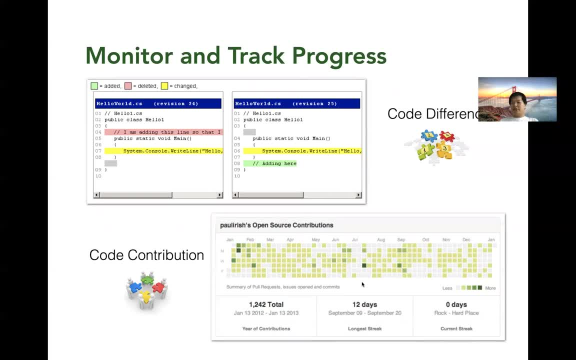 verify it's true or not, but you know it just means that most of the cases you didn't do it, or even you did it, that you're too irresponsible, you're changing. whatever you're doing, you're not following the right rule. okay, So that's some kind of executes you know nobody like. 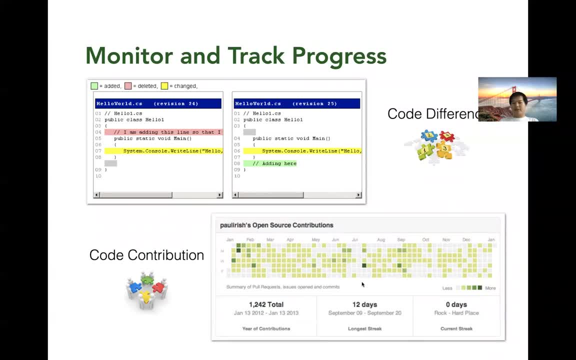 to hear about. all right, So just don't bother. You can think about some other execute, but that's a very bad idea to say: oh you know, I checked in, but it's actually under my teammate's name for whatever reason. okay, It's just very. 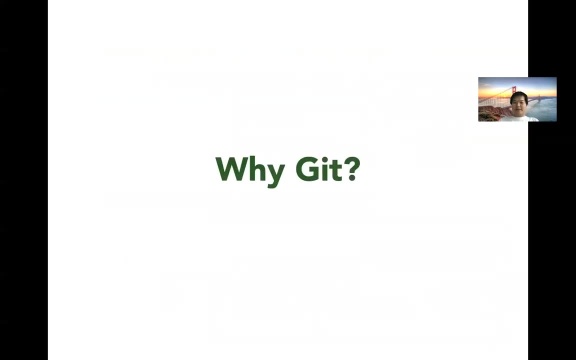 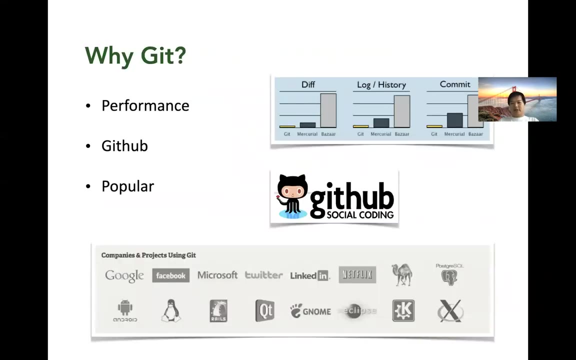 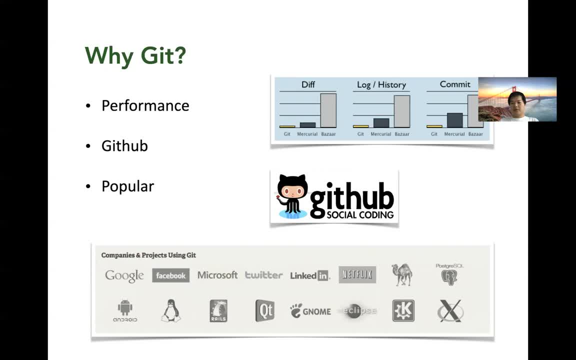 in 2011,, when I was doing the internship, Amazon was using a version of the tool, a version of the tool called a Perforce, and you can still search and find. it's a commercial tool called a P4. And Microsoft was using something called CodeDepot. It's a tool developed. 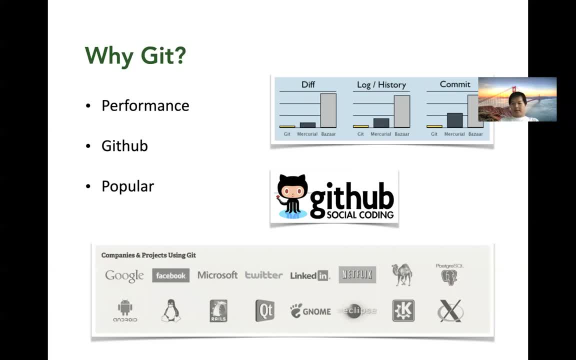 by Microsoft itself. It's not really released to the public, And then different often use different tools. There's SVN- some of you probably have heard about that. there's a, as then in, embedded in windows. that's was also very popular. however, after 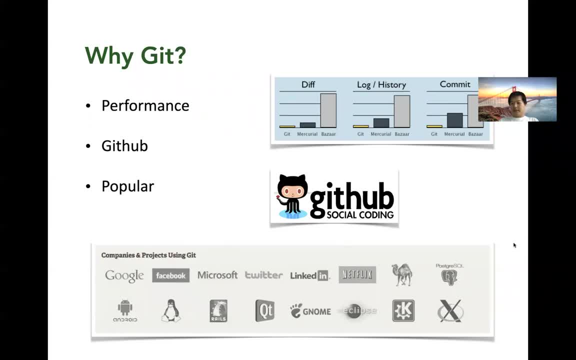 get shows up and pretty much everybody uh, started to use um, started to use get- okay, i don't know the exact account, but even the big companies they also started to get all right. so it's a, it's a big trend, very, very popular too, and simply because it's really performing really. 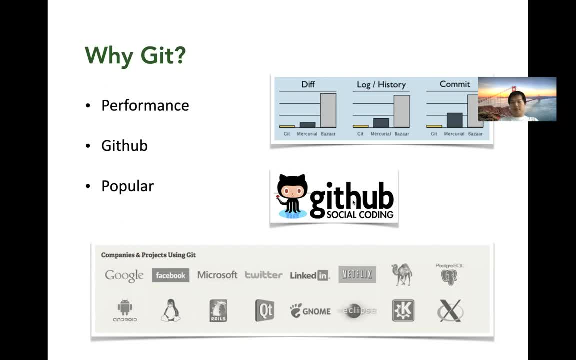 good. and then two is very easy to use and also, uh, i would say that github also did a good push to make this tool even more popular. all right, github just built this kind of social coding cloud hosting for other repositories. it's such a successful startup. okay, the company was acquired by. 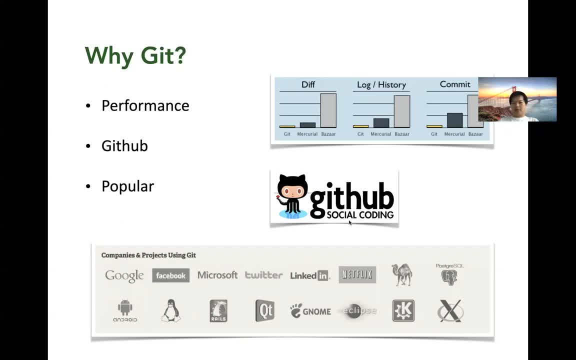 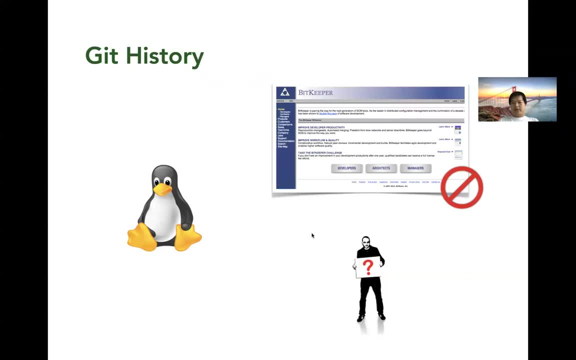 microsoft for how many? four billion dollars or something like that last year. all right, so very successful startup. all right, a little bit history about get you know. uh, it all came from this linux. you know, you all know that linux is a open source software and everyone can get a copy and can make some changes you can make. 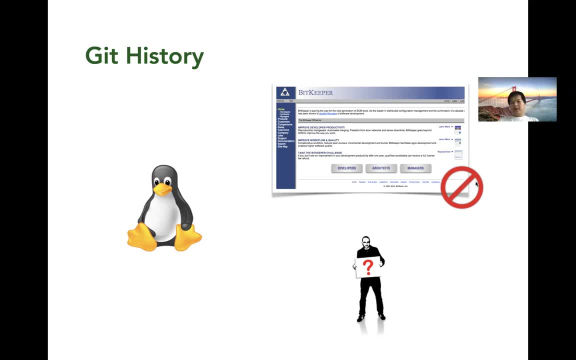 your own distribution of linux. in the early days, linux used this tool called a big tracker keeper. okay, for the version control. this is a commercial tool and i forgot the detailed story. i remember something about the license: that the linux team cannot use this tool anymore. something about that i don't. 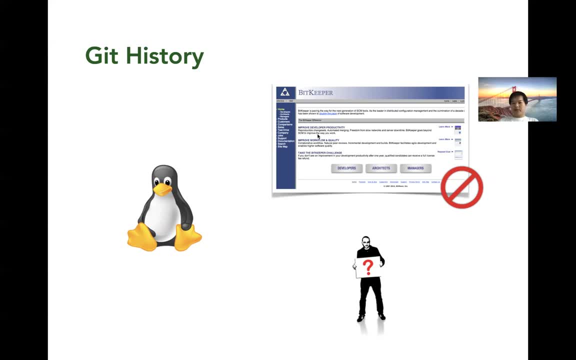 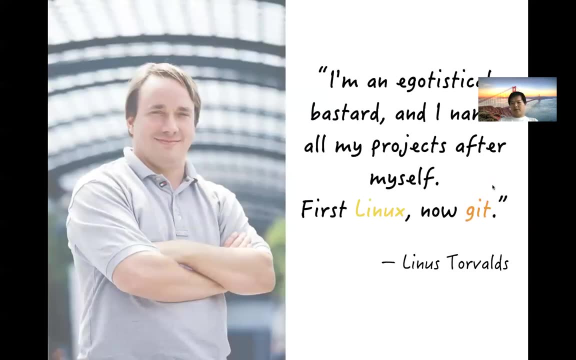 know why. i don't know why. because they they stop supporting it or they don't give free license, or whatever. uh, they can't use this one anymore. all right. so the author of linux decided, though, i will just write my own tool. all right, i'm not gonna use yours. 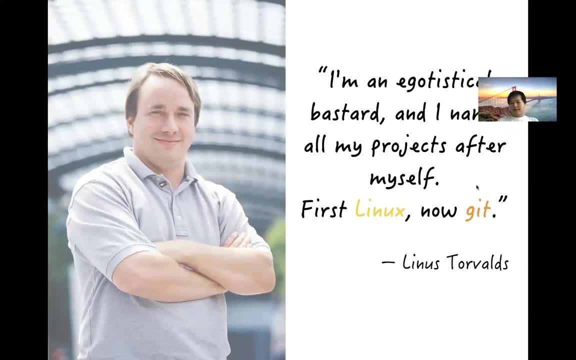 all right. so this guy just basically created git and he just did it by himself, um, and then that turned out to be a really, uh, popular and, um, famous tool, so he only wrote this to his offer in his life and the boats are super, super, uh like, uh, significant. all right, in terms of the 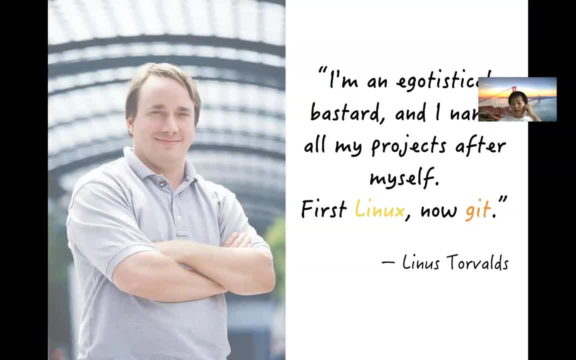 impact. all right, so that's a little bit history about git. so git is a very new tool. it only came out in 2006 i think, but it just grows so much popular and because, if you look at a vertical tool, there are so many choices before that. 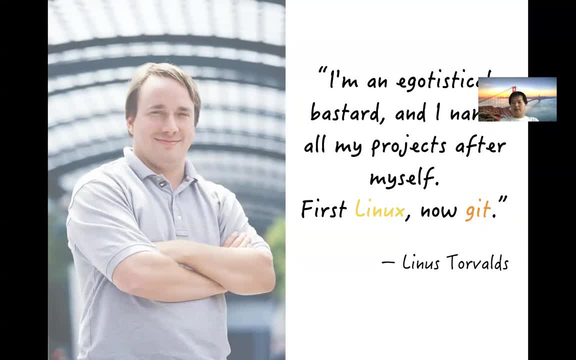 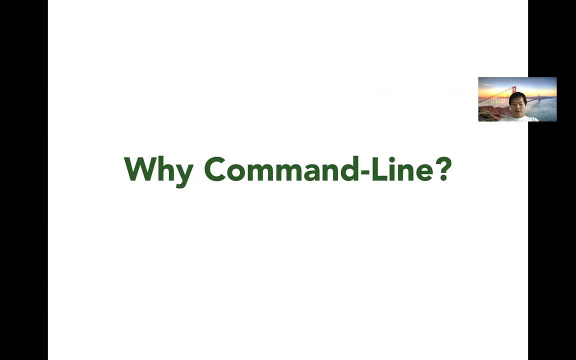 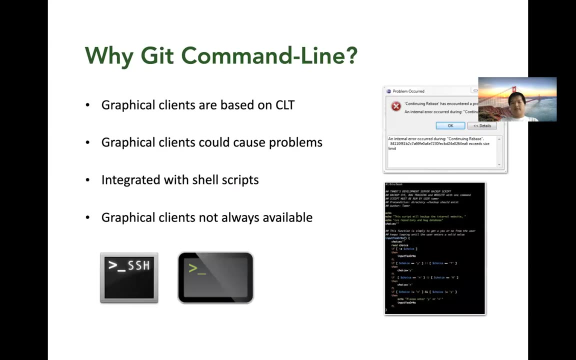 and then none of the choices you know dominate the market. but right now it's all about it all right. and when you are using git- i'm not sure how many of you are using the graphical ui. i highly recommend you start to use the command line all right, just because. 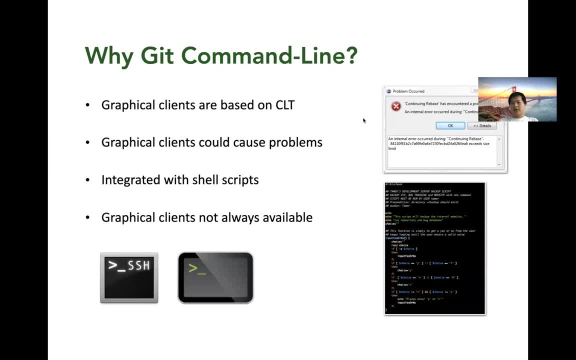 a lot of the heart. the graphical ui is not really easy to use. sometimes it is very error prone. if you want to do something very complicated, there's a lot of potential that you can get errors and it's very easy to debug and not very easy to debug. but also 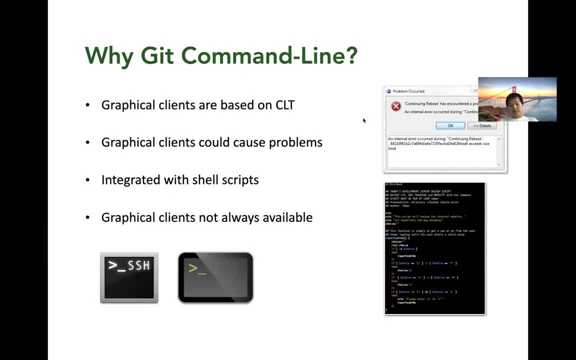 in the professional world when you have all the servers and you run things on servers, you don't have the ui to use. all right, so you have to rely on the command line. but also, you should know, a very big benefit of using the command line is you. 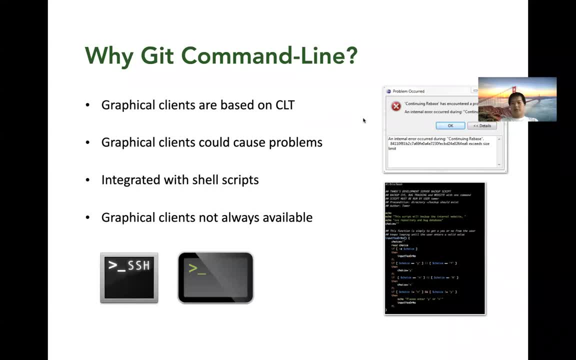 can integrate those command line to some of the scripts, all right. so this happens more when you do a lot of software operations- the server operations and maintenance- that you need to have certain kind of script to do certain tasks: to automatically deploy the software, automatic clean up the. 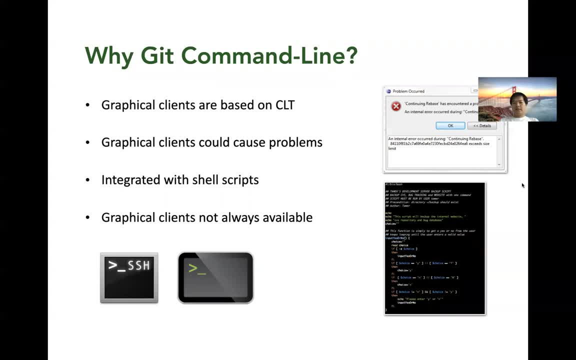 logs all of those and then the command line will be the only way to go, because you won't have this kind of ui to help you. all right and um, yeah, so after that, and you know, yeah, as i mentioned, sometimes you just don't have the graphical client. 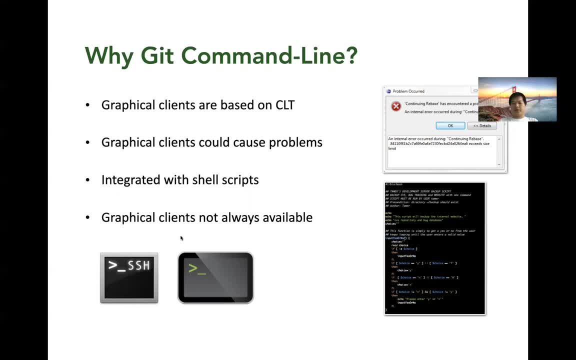 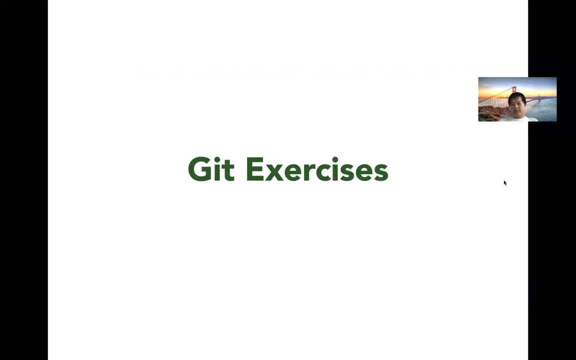 available. all right, so as a cs major, you should actually start to use the command line tools. all right, so for the git um exercise this. all right, so i i don't want to show too many. uh, it's really simple. i'm sure some of you haven't really done this much. 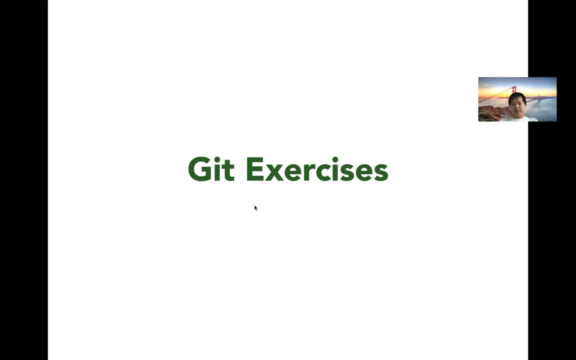 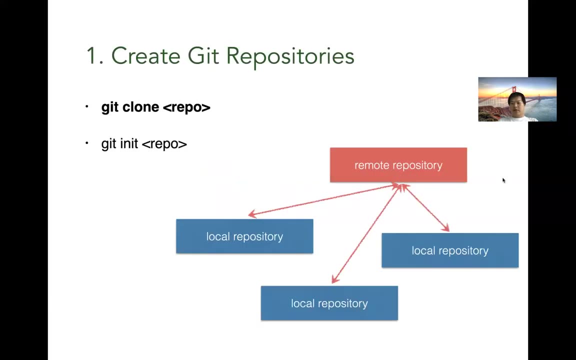 but, um, my recommendation is, after the class, take a look at some of the tutorials about git and you can find a lot of good resources. all right, so i'll go through some of the very basic uh concept here. all right, so, number one, you need to understand the repository. okay, the repository i already showed you. 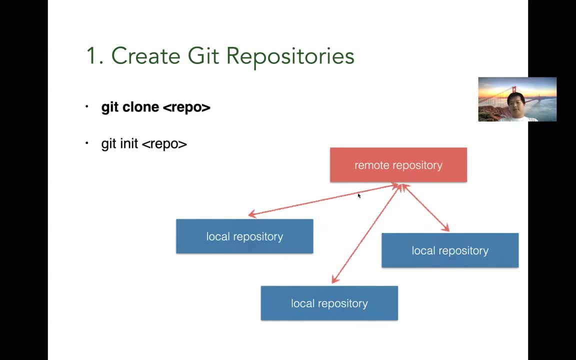 in the bob and alex as example. it's basically centralized code copy. now the the way git works is that: um, every time when you are working on making some changes, you need to first get a complete copy of this report. remote repository. all right, this is different from some. 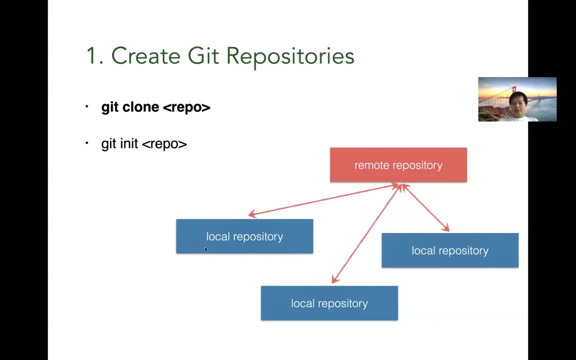 other tools. the copy you get on your local computer is exactly 100, the same as a remote copy. all right, it's not a partial copy. some older tools that they only have a partial copy, but git just allows you to not allow you, but just require you to. 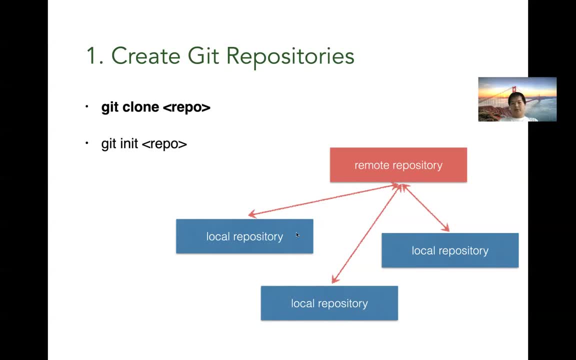 get the full copy so that you can get every information. you can just do it totally independently your local environment, that's how they do it. so the very first step you need to do is always to clone the repository from existing uh repository, right? so let's actually try to show some examples. 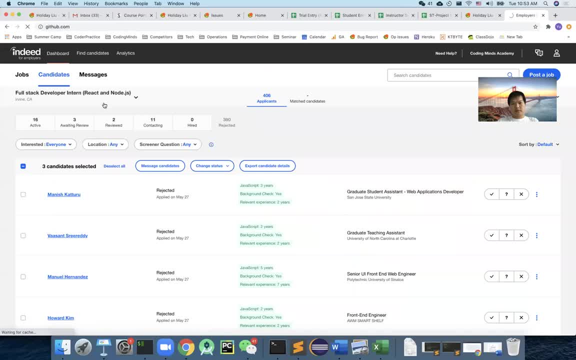 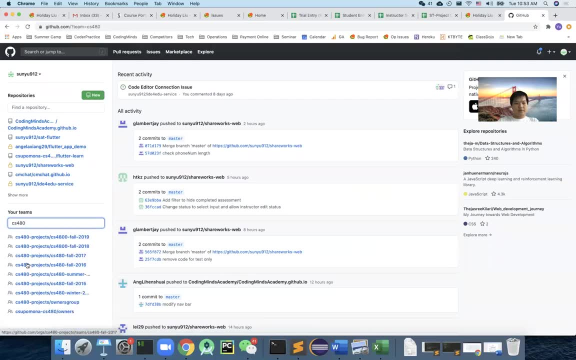 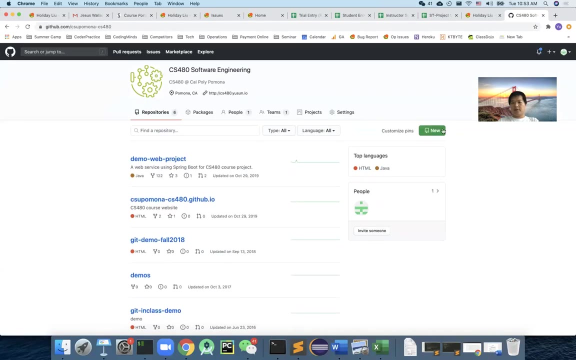 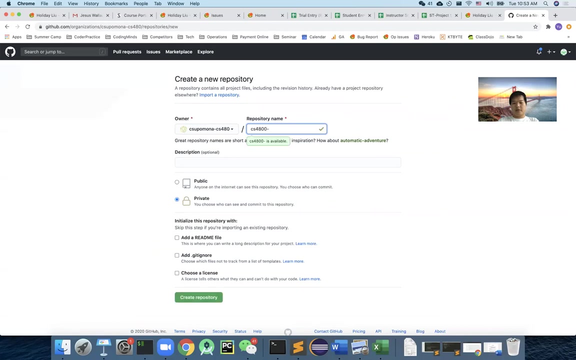 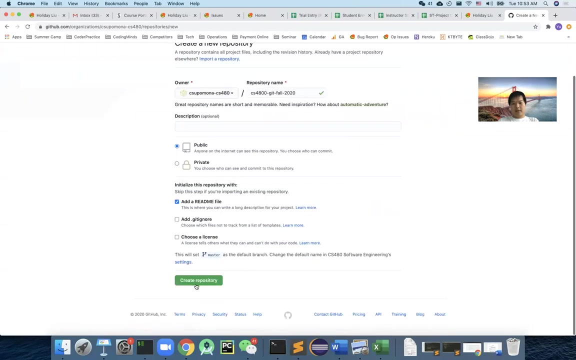 all right, so i'm going to go to github, all right, so let me actually create a demo repository. so let me create a new one. all right, so i'll do something called uh, cs4800, git and fall 2020 public. i'll add a reading file. 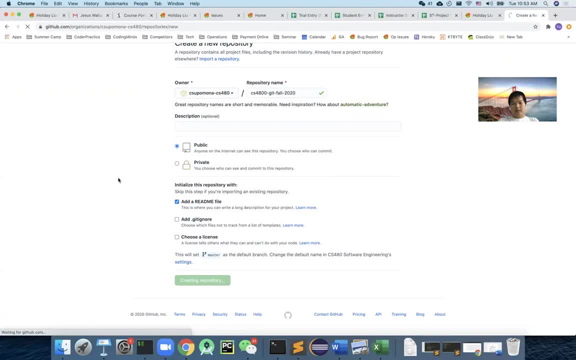 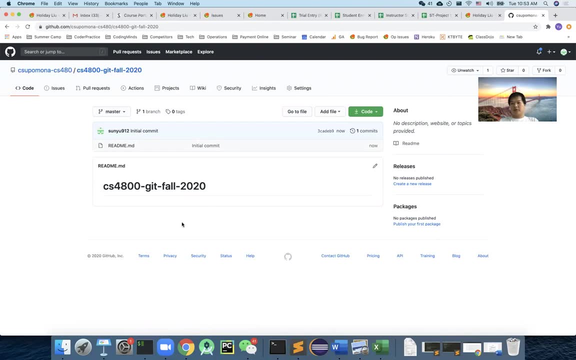 create a repository, all right. so, um, if you use github or some other tools, you can just create your centralized copyright here as your host. obviously, you can also host your own github server, but you don't need to do that. github just does everything for you already, all right, so this is your centralized copy. now, if i want to make something, 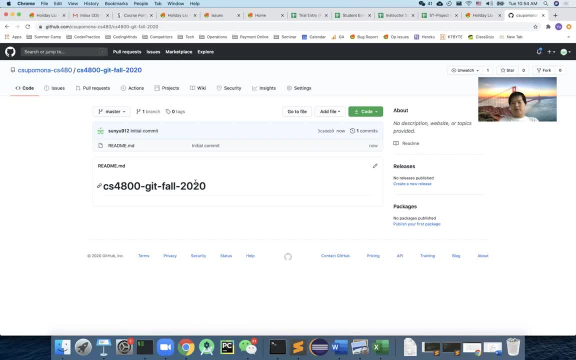 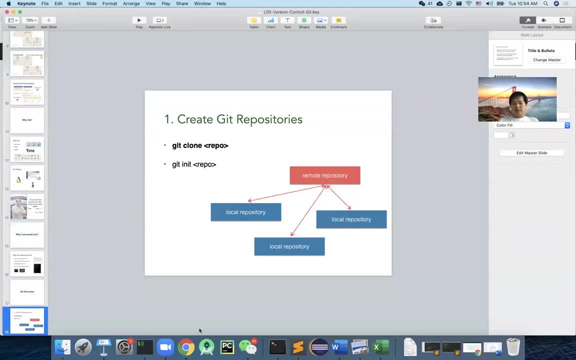 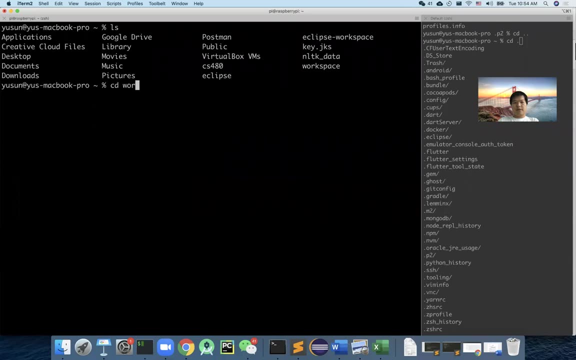 changes. i just need to get this copy to my local computer and then work from there, and then to do that you will need this command called git clone, right? so i'm going to open my terminal here. all right, so i'll go to my workspace- funnel folder. 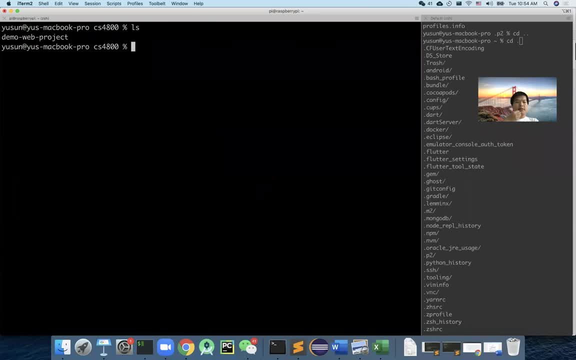 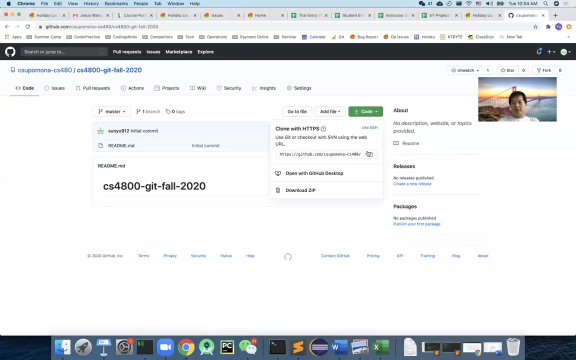 i have a 4800, all right. so there is one project, that's the web service project, all right. so i'm doing a command called a git clone and i need to specify which repository i'm going to clone. so you click on this button here. you get this address. 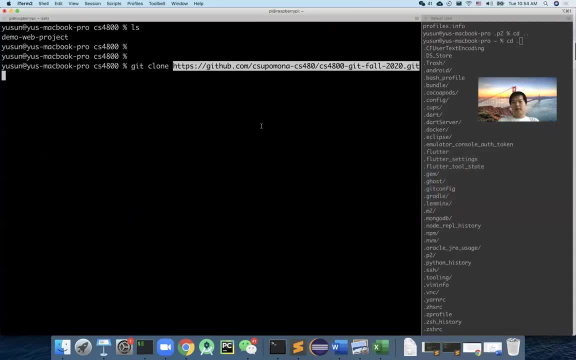 and then you copy it over. all right, that's the address server to your repository. i hit enter and you can see it just quickly. download everything, not many files. and i do the file folder again. i can find out this little uh folder here. so i get into the folder and there is this one file called. 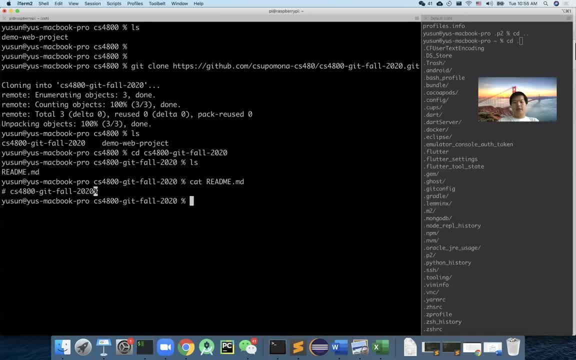 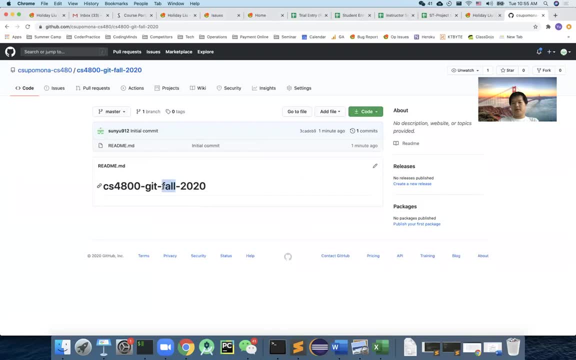 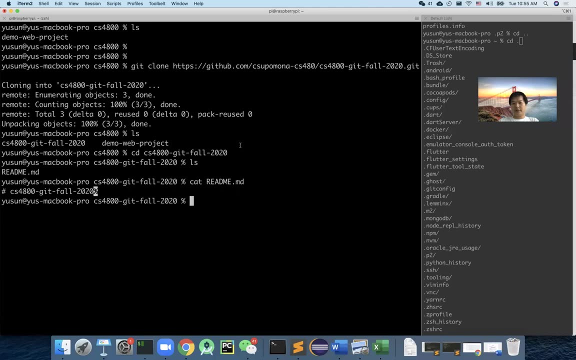 review file and you want to see what's inside the reading file, is this? just one line of code, the title, which is the same as the one you see right here. all right, but by doing this one, i'm actually getting a local copy of the repository from github, which is the host, all right, and this copy is exactly the. 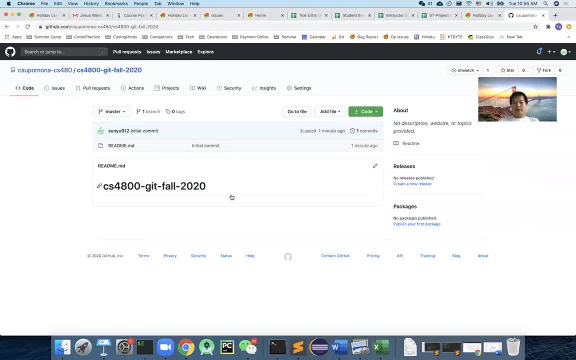 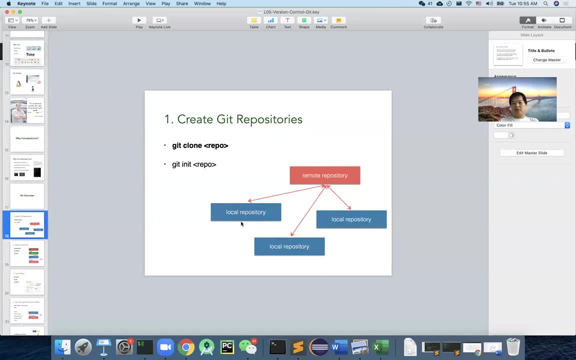 same as your remote copy right here. so that's how you actually start to work with git: just get a local copy first, and all the changes you're doing you go to the local copy first. all right. so after that then you need to know how do i make some changes, how can i make some? push my changes to the 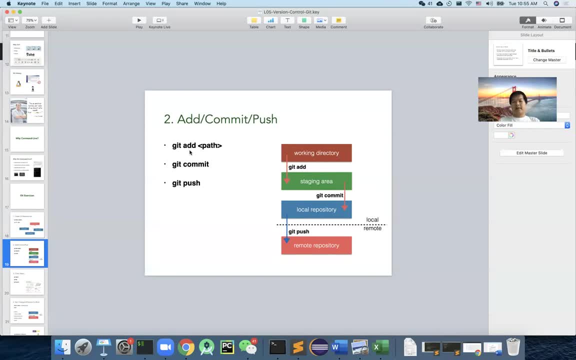 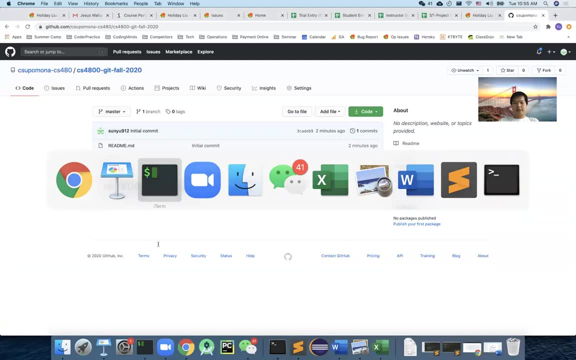 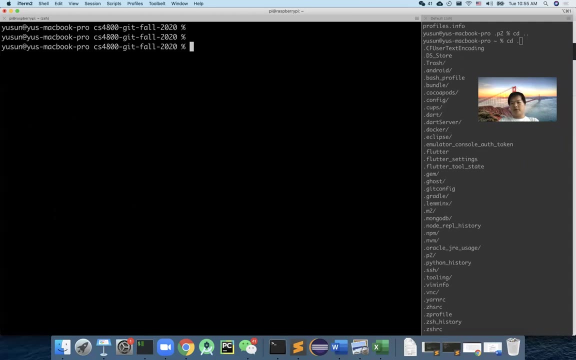 remote repository, right, so you do a few command called add, commit and push. this represent different kind of steps, all right, so let me show you this, this um so, once you get here, all right. so, uh, before i show you the adding, you need to know something very important. 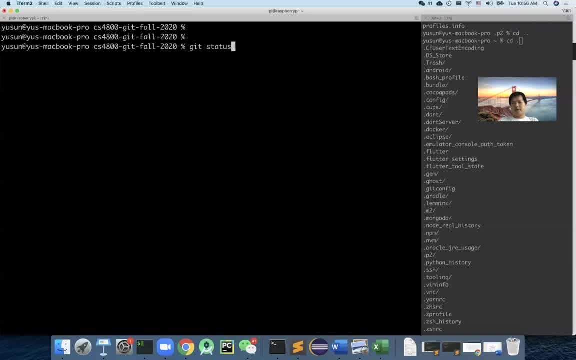 command why it's called a git status. right, so the git status is your friend, okay, so it's really helpful anytime when you are in the git repository. all we use the status to try to understand what's going on right now in the repository. where are we and what's the status? what are the things i need to do are? 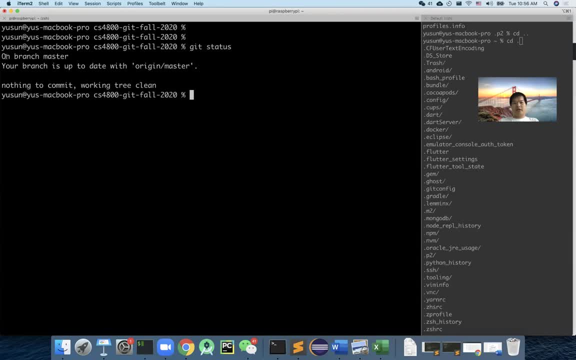 there any issues? so right now, this one just shows you: okay, you are on the branch master and it's all up to date and nothing to commit: working tree coin. so looks like it's a very good status, all right, and then. so let's make some changes. 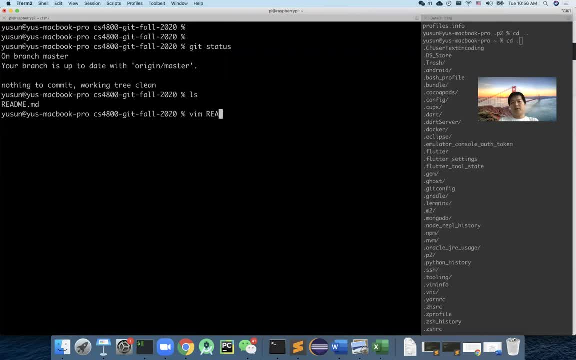 all right. so there is a readme file. i'm going to make some changes just on the readme file. open my uh, just uh, i'm going to do a vm to do some changes, all right. so i'm doing something like: uh uh, you know, section, uh, copy one. 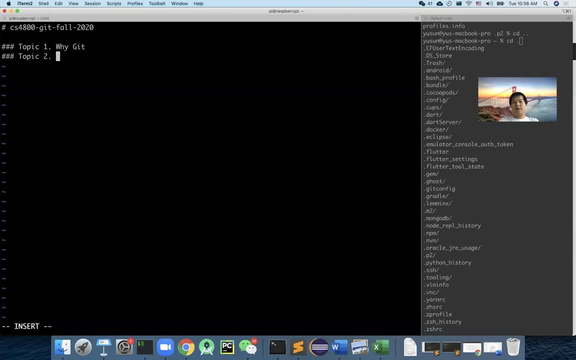 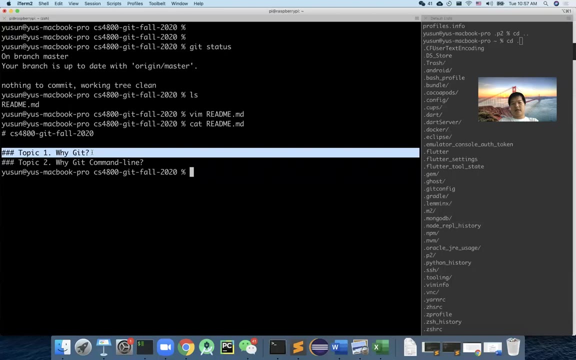 it. copy two, y, get all right, so make some changes, and then i'm going to save my change right here and right now. if you look at my file, i have some extra content, But this content only sits in my local copy. If I go back to 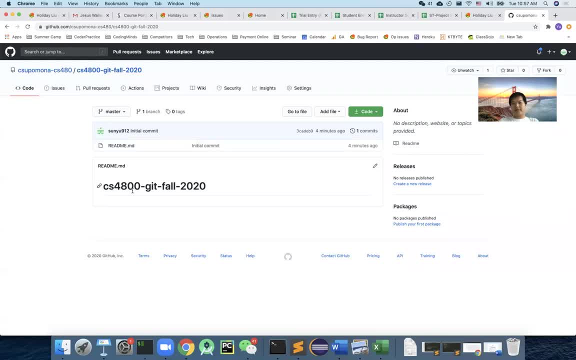 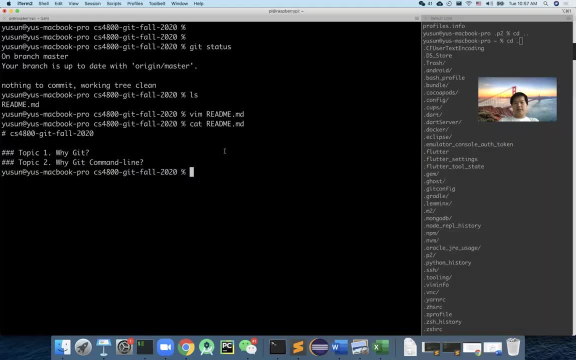 here I refresh, and this one doesn't change. So what I want to do is I want to push my change from a local to the remote repository. So there's a few steps. Number one: let's try to get status Now. as you can see, it says that: 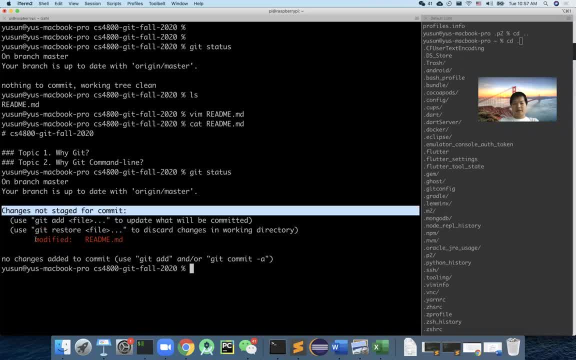 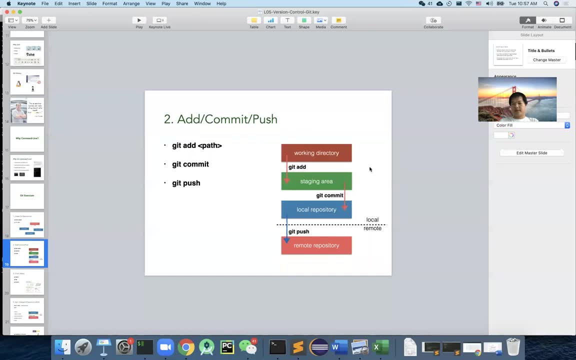 change is not staged for commit And then there is one file here that says modified: All right. so that's why you need to understand some of this kind of a different little stages when you are working on some changes. So we're right now at this, working directly, we're making changes, And then you can do. 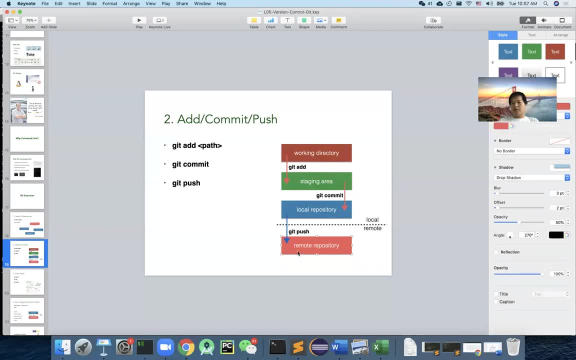 any kind of change you want. It has nothing to do with the remote repository, But the moment if you decide you want to push things to the remote repository, you have to go through the two extra steps. One is you have to confirm what are the changes that you want to add to the next. 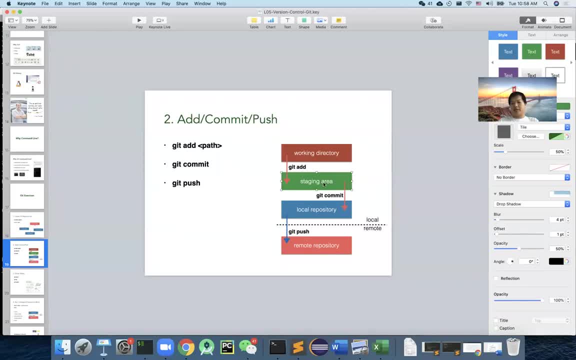 version. We call it putting that into a staging area. Once you have a bunch of changes in this area, you're good to go. Then you create and one commit to include all those changes And then finally you push that one to the remote. 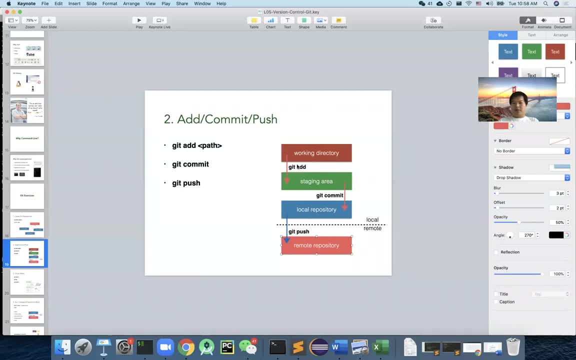 repository, All right. so the reason to have this one is to this step is for you to identify what are the changes I want to push and what are the changes I do not want to push, Because there might be some kind of testing you do in the 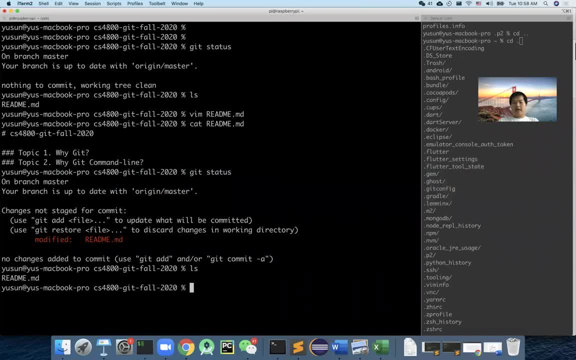 folder here that has nothing to do with the final change. then you don't have to have the repository to manage that. You don't want to have to get to remote to monitor that, So at that time you don't have to do the staging. So let's come. 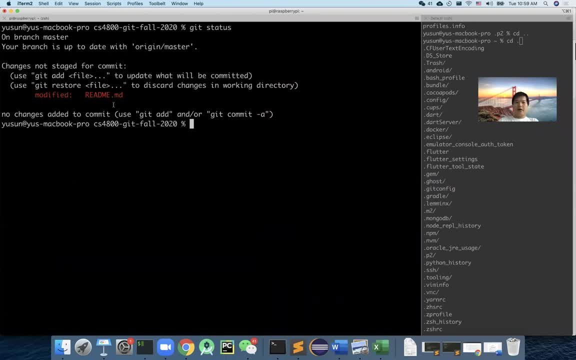 back here. Let me show you this again: Get status. This is the file being modified and I think this is the change I want to push in eventually. So I do git add and I do this file name. I want to add this one to. 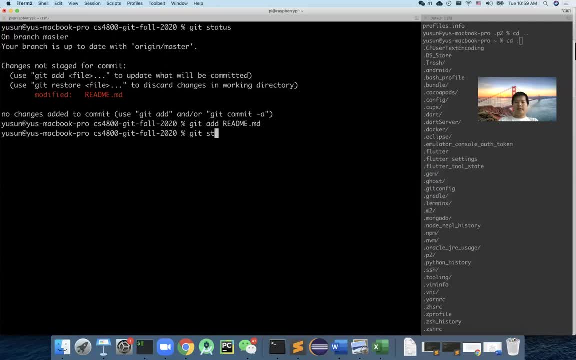 the staging area. All right. so now I do git status and you can see it says changes to be committed. So this means I already confirmed that this file will be show up in my next change or next push. All right, so I already kind of added. 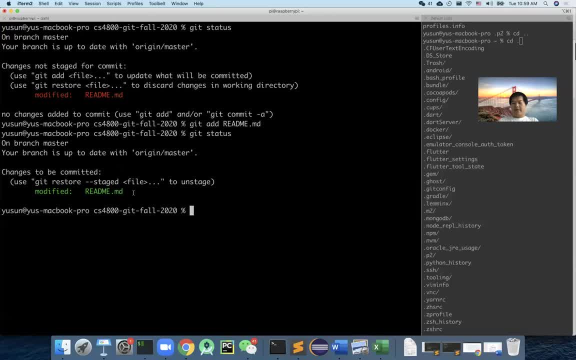 it here, so it's green. And then you might have a lot of files in this kind of a stage, because one feature change is not often not just one file. I have multiple files. So at that time you can say, okay, I will do some. 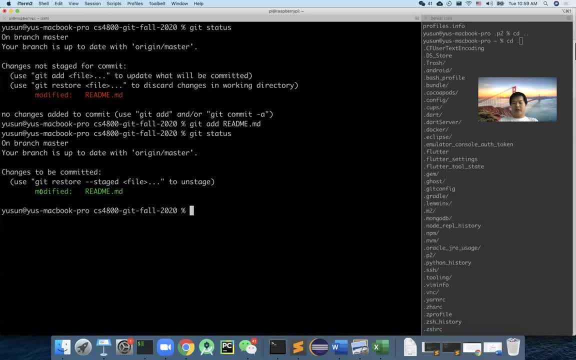 other changes, but eventually I'm done with my changes. I want to push, I want to send it to the remote. This time you need to do something called git commit, All right, so you commit one change to the remote server Once you hit this. 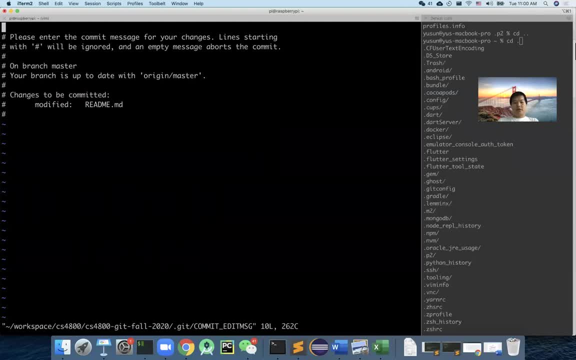 command. it automatically opens the code editor From your OS. If it's Windows, it will probably open the notepad. So this one asks you to type some kind of commit message. This is very important, So you want to show and type what you're changing and what's the purpose of the. 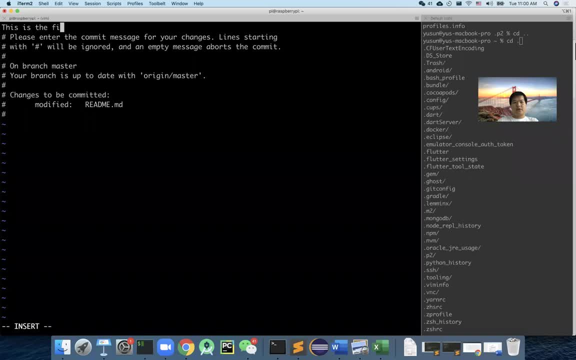 change. So I'm going to type something called. this is the first push I made: Yeah, 4800.. All right, just to describe briefly what you're changing And what's the purpose of change. So save this one and then you're done with. 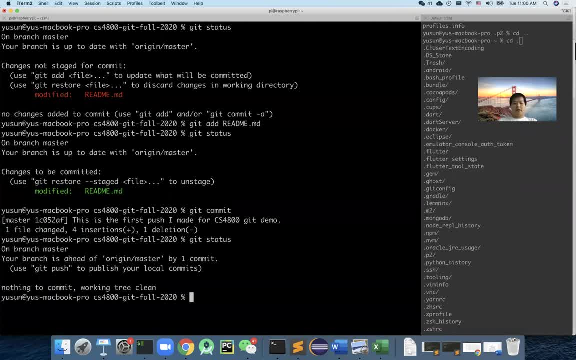 this commit. Now I do git status. All right. so you just finished kind of a local change and that's called one commit, And then they said that your branch is ahead of original master by one commit. So that means right now this callback I have in my local computer is ahead of this one here, because this one 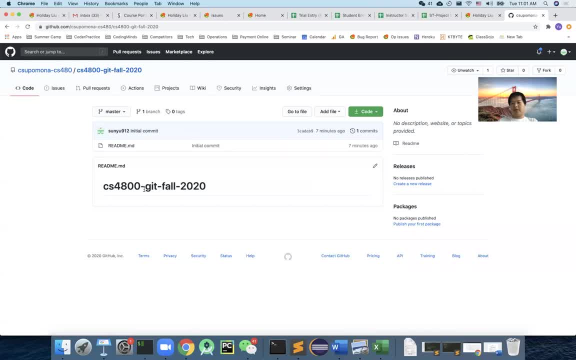 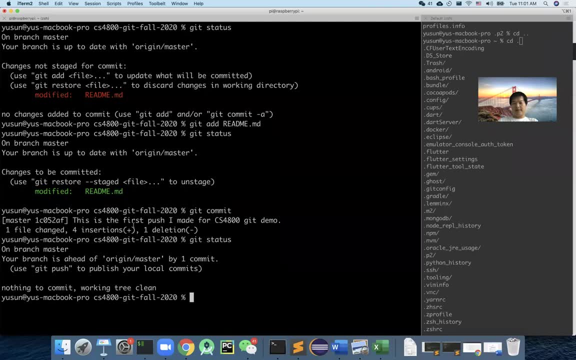 still doesn't have this change I made recently. But then the local copy knows it because I made a bunch of changes. I made a commit and now I'm adding things on top of it and it has more things than the remote server. But again, this is still only sits in the local and that's why. 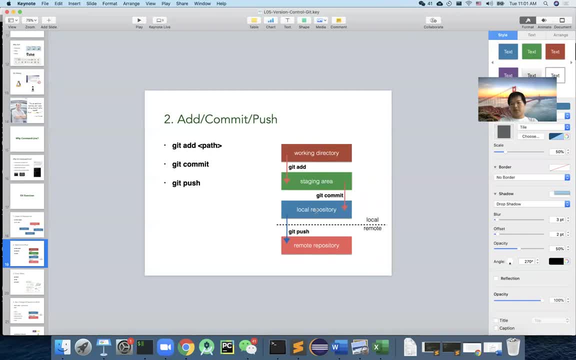 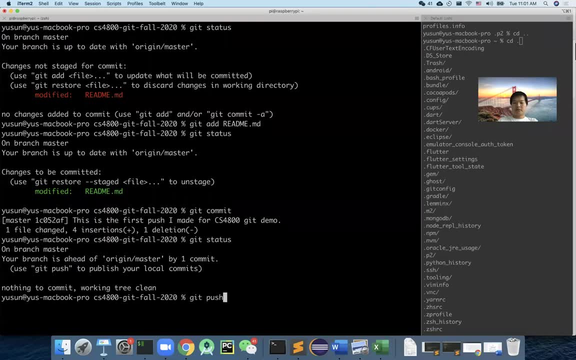 it's actually here called a local repository. I made the changes to the local repository not here. If I want to do one more thing, I'll just do something called git push. All right this time, as you can take a little bit longer, because we're. 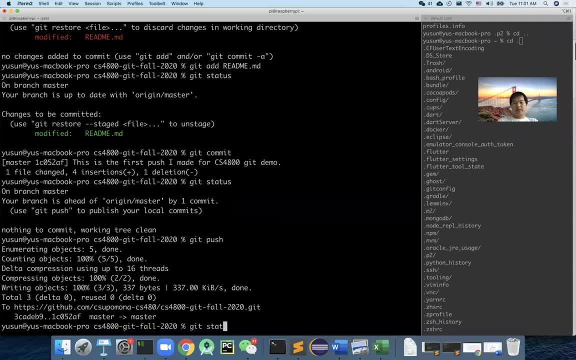 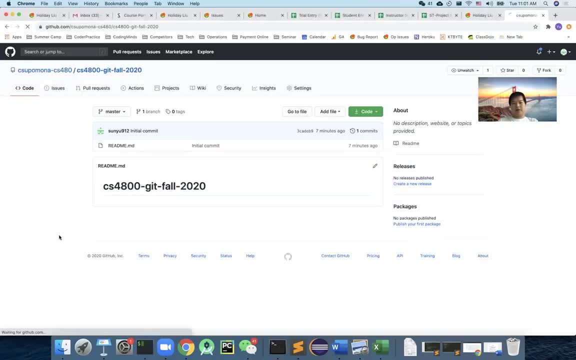 uploading the file to server. After that we do git status and it come back to the clean, up-to-date version. And now, if I go back to the, to the browser, I refresh. All right, so, as you can see, we are adding these two things into the streaming file. 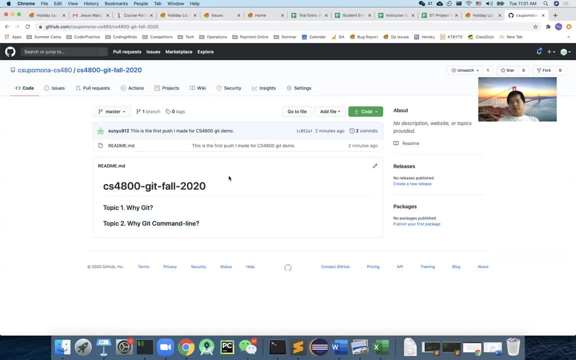 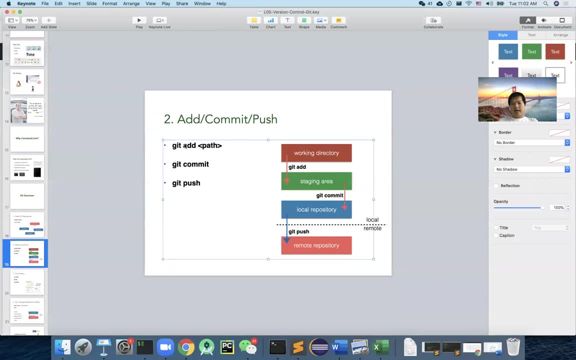 All right, so that's how you completely pushing one change from local to remote repository. All right, so it's pretty much this: four: command, Add, commit, push. All right, just this once, Let me see for any kind of questions here. Oh yeah, for. 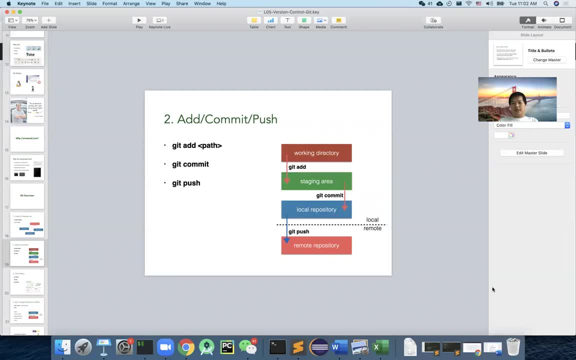 license. it's all up to your choice, right? because if you want to open source that and you can- you can pick it. The difference between different lessons is how you, how much like a rights you gave to other developers. if they reuse your code, Can they commercialize? 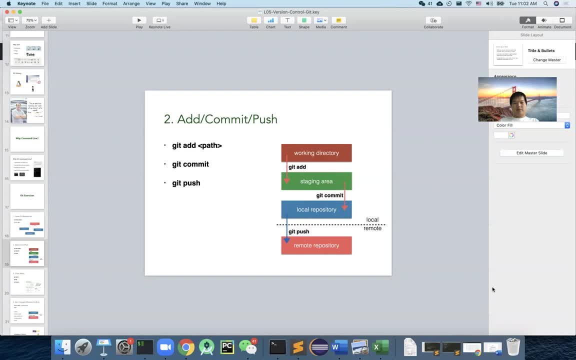 that? Can they actually publish that or whatever? So there are different license that give you kind of some. some of those are very like a phrase. Some of those are very restricted. So it's your choice. You can take a look at the differences. 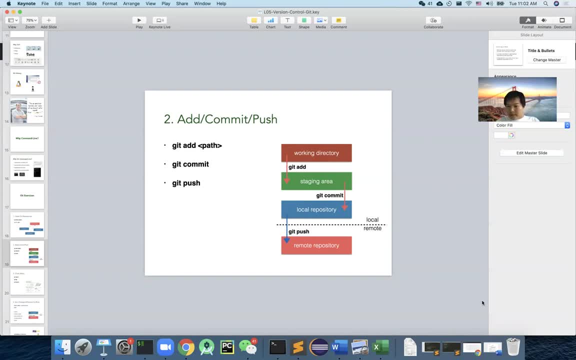 between the license. All right, let me see some other question here. We have two folders, one server and the other kind have had a lot of combining this. So are you talking about like initialize and existing folder into GitHub? Yeah right. 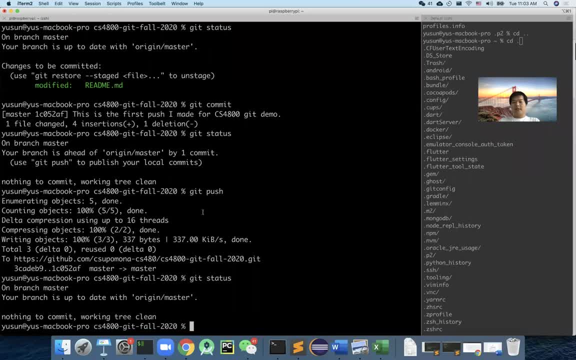 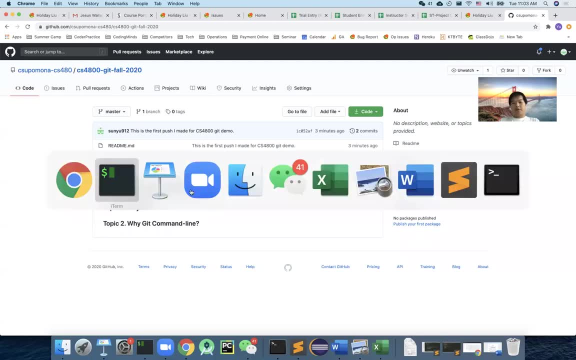 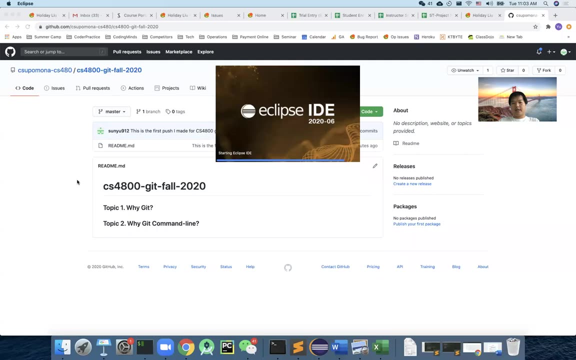 So I have some good practice with that one. So the way I showed you give clone is something you already create from here. That's all. would recommend it, But also a very common case. is this All right? so let's say, I go to Eclipse, I have one project there, All right. 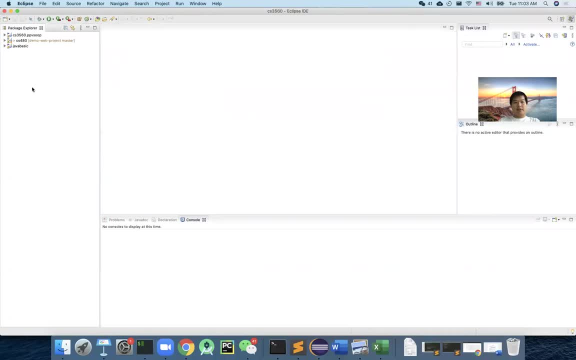 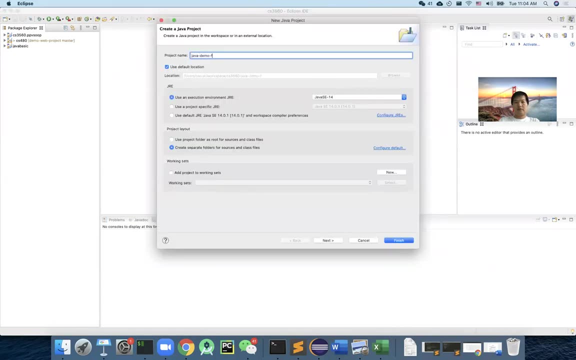 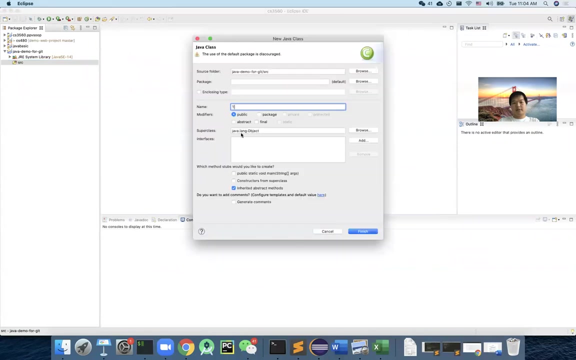 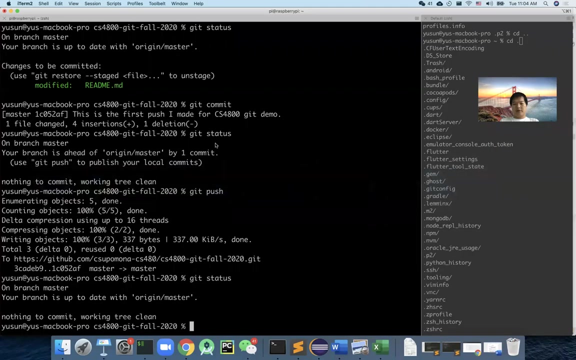 All right. So let me see. So let's say, I create a new project, It's a Java project, All right, And then I can create a new class, All right. so I did something, But initially I didn't really do anything on the repositories. I didn't do that version control, And now 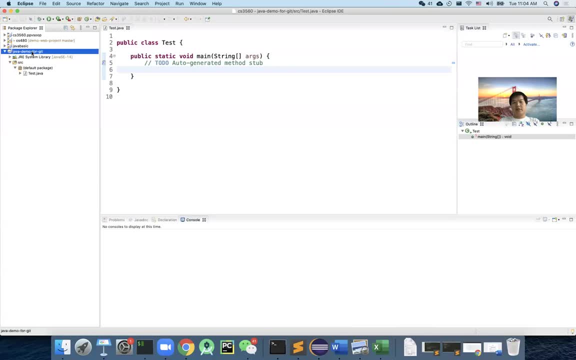 I decided this project, I want to save it, right? But it's not really a good project. So this means that you want to create this local copy and then make it at the remote repository, Right? So you want to create this local copy and then make it at the remote. 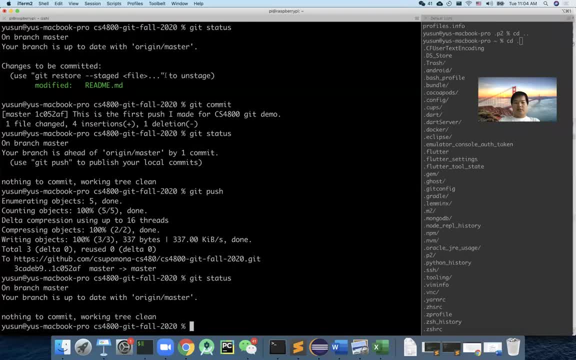 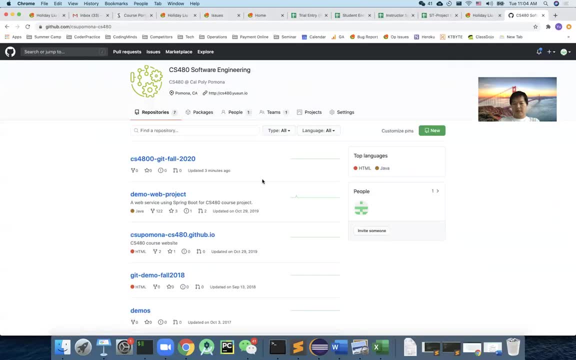 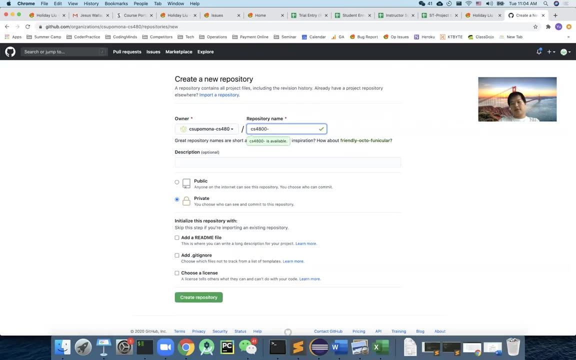 repository somewhere in GitHub, for example. All right, To do this again. the same thing. The best way to do this is you go to GitHub to create one repository first, So I'll create one called cs4800.. All right, I'll do a. get demo Java. All right, make it public All. 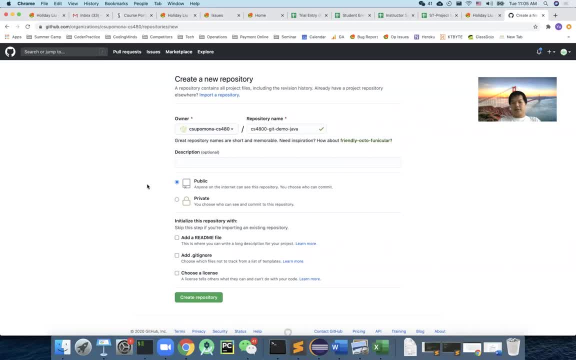 right. So again, this part is very important. If you have this kind of situation, the best way to do this is: don't create a repository, All right, So I'm going to create a repository. All right, So I'm going to create a repository, All right. So, again, this part is very important. 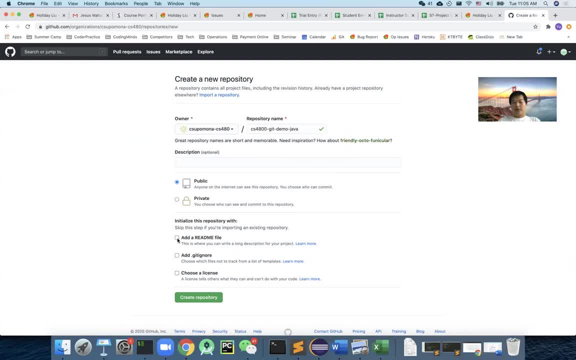 It's like if you have a data, don't initialize any of those, because the moment you create a file there, that means this repository already have something, But then if you don't create it, then this repository has nothing there. When this one has nothing, it's a little bit. 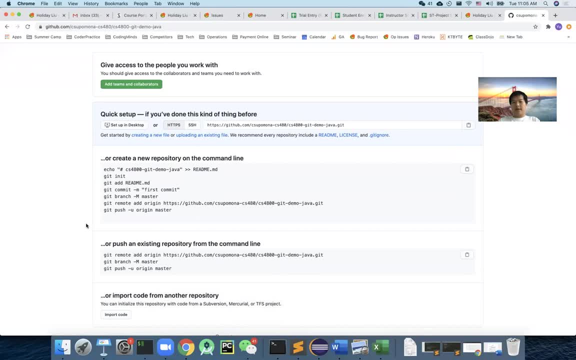 easier for you to adapt some of the changes to this one here, And then I really want you to pay attention to this command. These are basically things you will need. How could you get local folder from your local computer and then push it to here and then keep your? 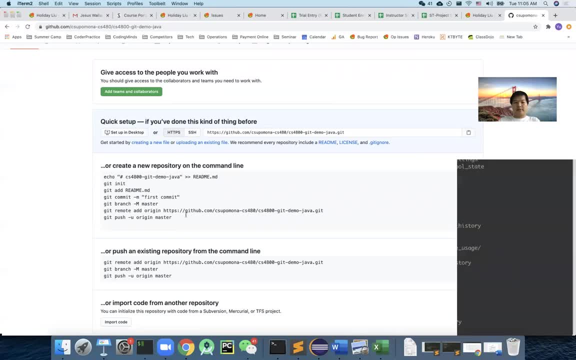 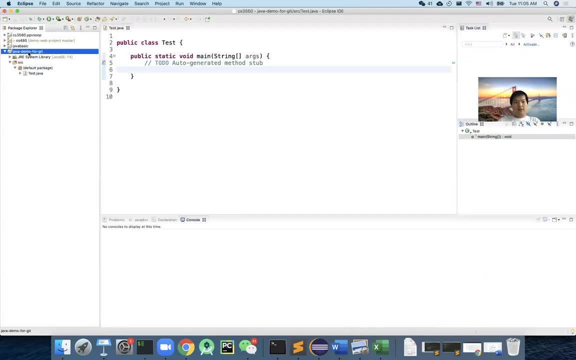 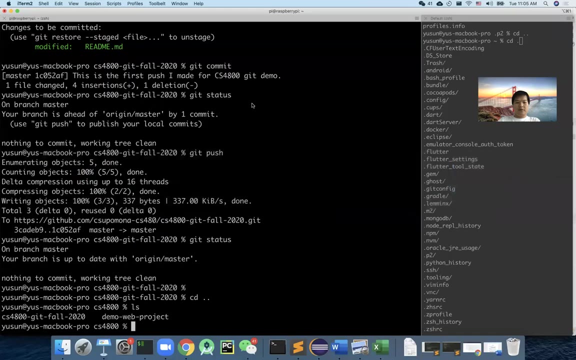 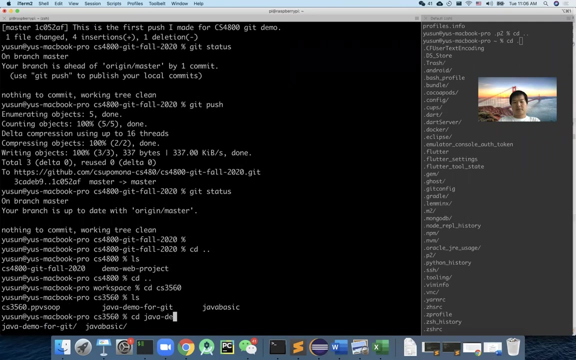 mind this command. this one shows you all the things you need. all right, so let's try this. so i'm going to find out. i need to find out this one first. okay, where this? uh, this one here. yes, okay, folder, right here. this is the photo. we just created the project. if you do a key to status. 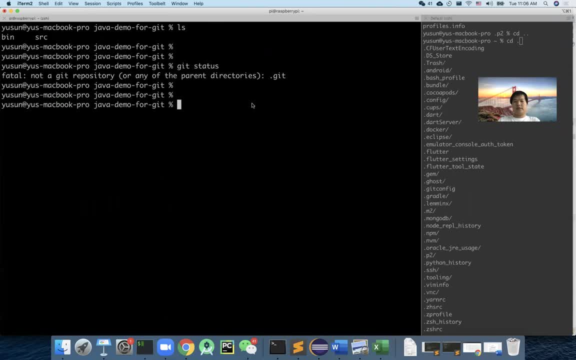 you can see, it's not a git repository, so it's not good yet right. so let's follow the steps here. okay, first one is called git initialize, but this way it will make this repository as a git repository. so now if you do get status, all right, so everything is fine, but then you're not really committing anything. there are some 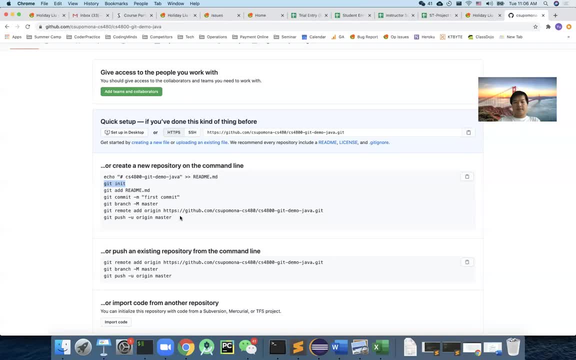 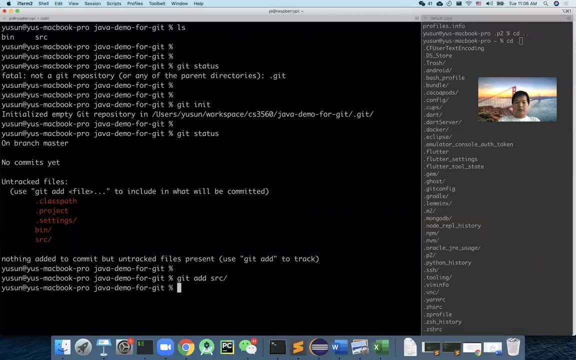 files here and then, but then you didn't check in any of those, right? and then you choose what to add. all right, so i'm going to get add, for example, the source folder. so i'm going to get add, for example, the source folder. that is what's mounted at. maybe something else like project settings. 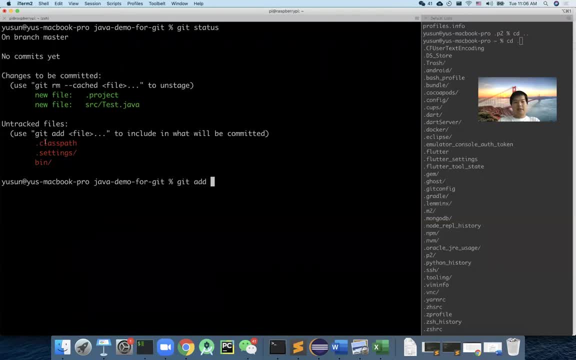 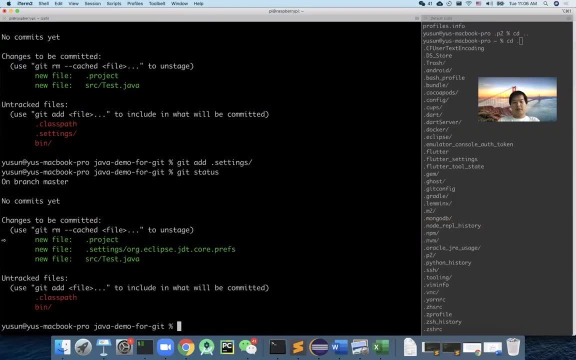 that is all we do: the status. i want to add maybe some other settings. this one shouldn't be needed, so i'll do a settings, all right, but i don't want to check in the bin folder or other folder. all right, so i confirm all the changes and then do a commit. so git commit. 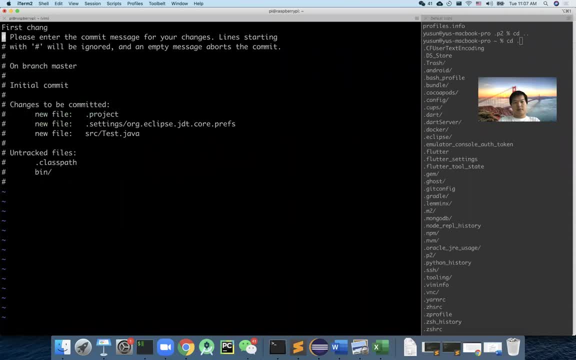 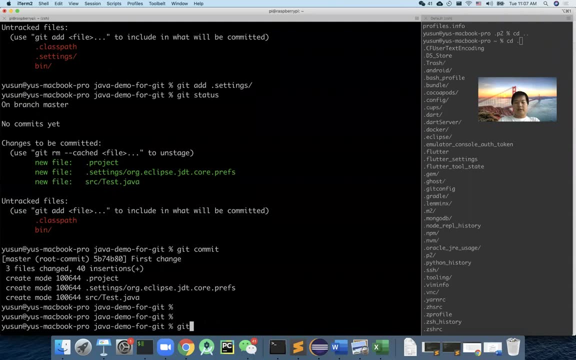 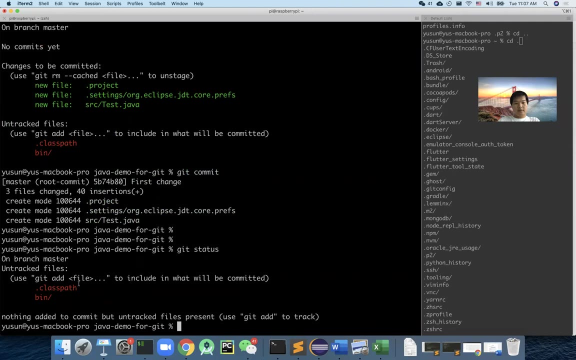 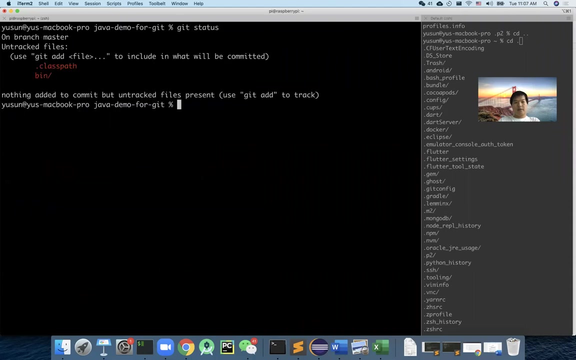 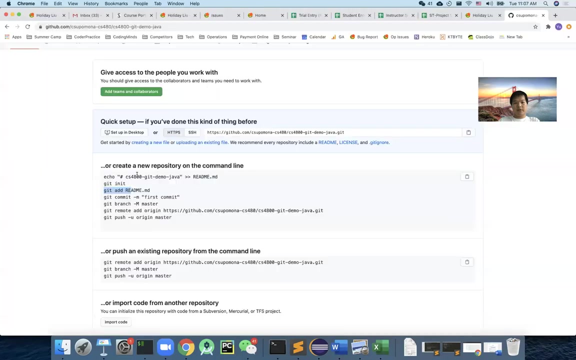 all right, so now git status. i got one commit here. we, sorry, did i do it okay, so this file is not tracked. but i have something to write to commit, Let me just keep going. And then you also need to create a branch called master. 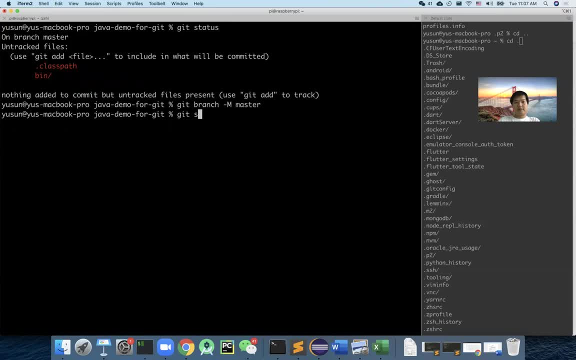 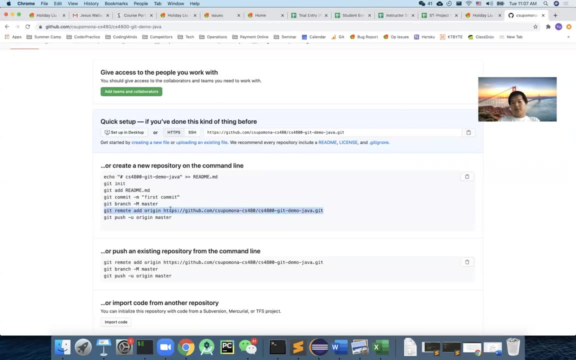 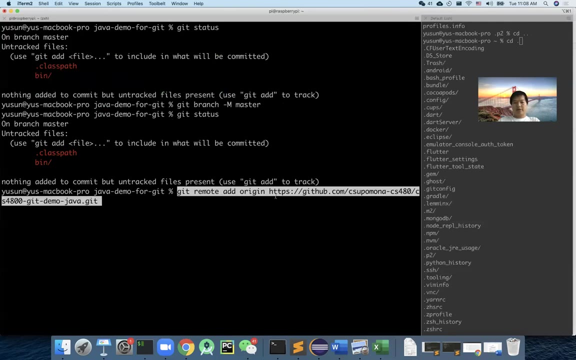 and let's just follow this command here. And then- this is very important- This is how you can add the remote repository to this local, because right now your local repository is not associated with the remote repository, So you add this one by adding the address, and now they're. 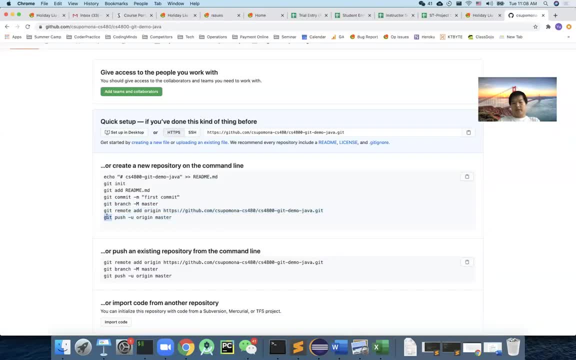 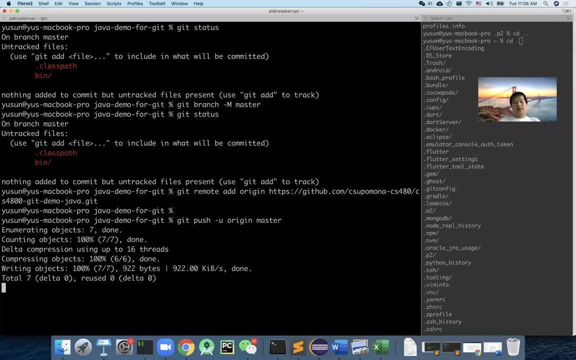 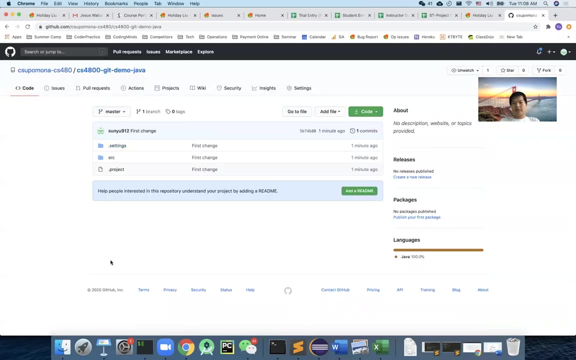 together And finally you do this kind of push command to push that to the order master. That's how you can get your things out there. All right. So now, if you refresh the repository and then you go to change it right here, All right. So this is the easiest way I can tell. 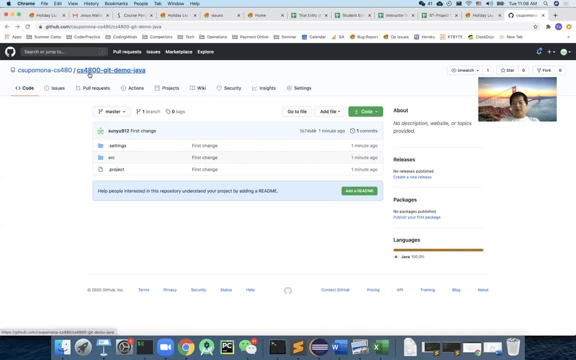 you. that's easy to follow. You saw this list of commands from GitHub. If you follow that steps, all right. However, if you do have something existing that you want to adapt to here, it's still possible. All you need to do is Google and find it. But you know that's. 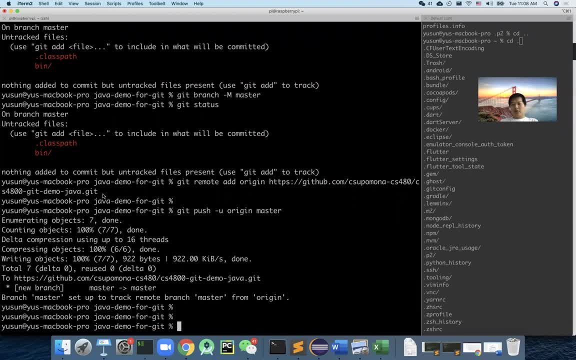 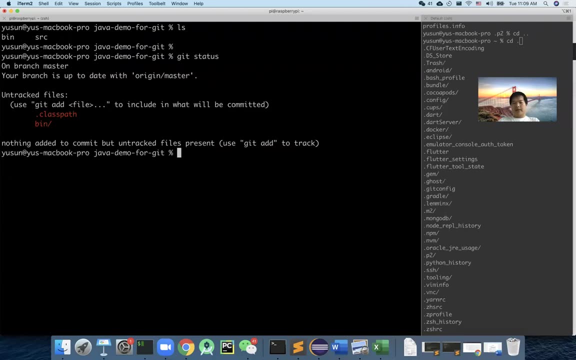 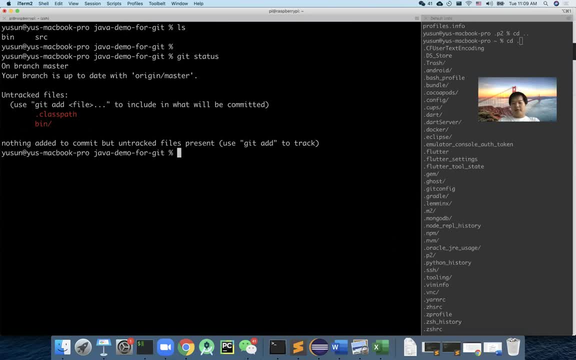 going to do this, All right. all right, what you need to do is back up your file first. Another one you can do is if you look at the folder here, if you show all the hidden folder, if this is the Git repository, there will be some folder called dot Git, All right. So if you go to dot Git, this, 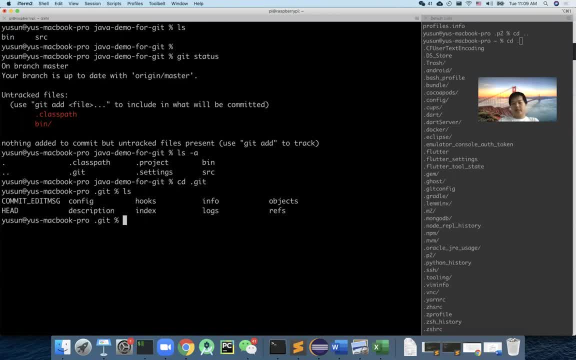 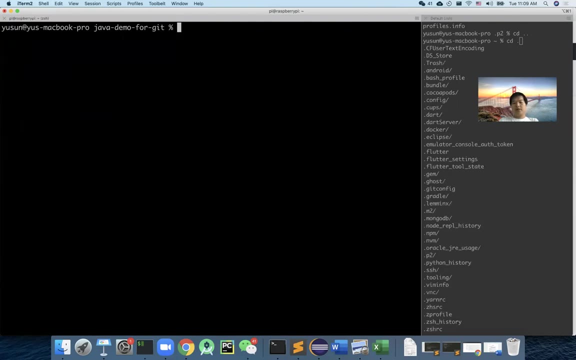 one has everything about this repository and then you don't have to attach. these files is managed by Git to itself. All right, every single history is managed and saved into this dot Git folder. Okay, So if you find this whole repository is totally messed up, all you need to do is remove that. 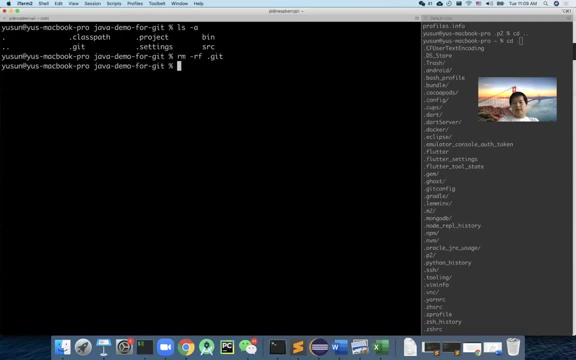 folder. So remove folder. All right, That's it. After that you look at all the Git stuff. it's not a repository anymore, You're not losing anything And everything is saved here. So this is a really nice feature about Git, because in the past the version control tool 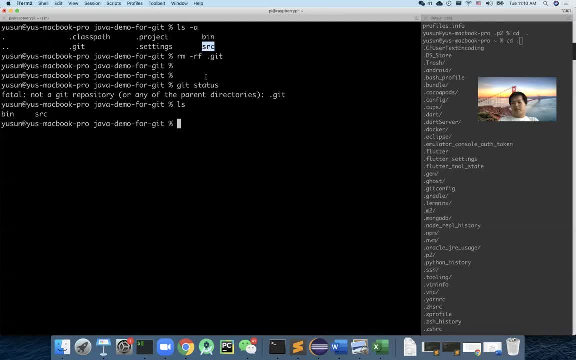 will put a lot of things into different folders and for various purposes, But now Git has everything in one folder. Now you clear it, it's gone And this is no longer a Git repository, then you can reset everything, redo everything. So it gives you an opportunity to redo it. 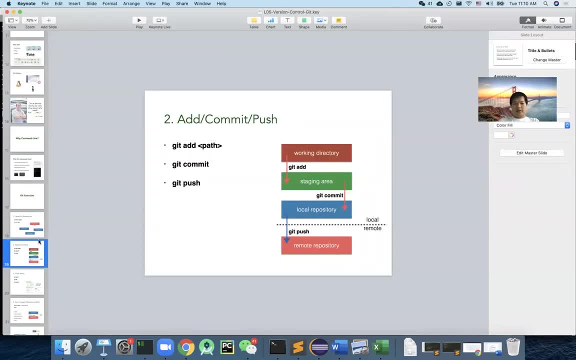 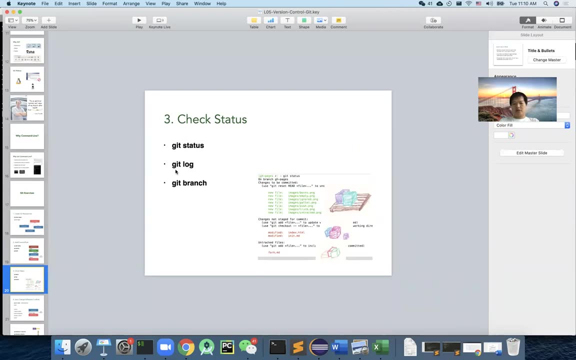 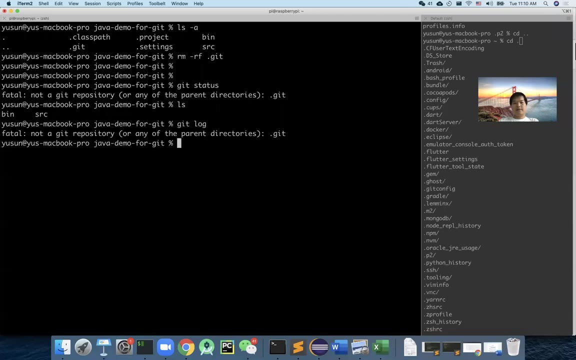 So that's something I want to mention here. All right, So that's how you add and also talk about some of this command: that how do you do the status, How do you show the log and branch The log means that if you go to here and you get log, 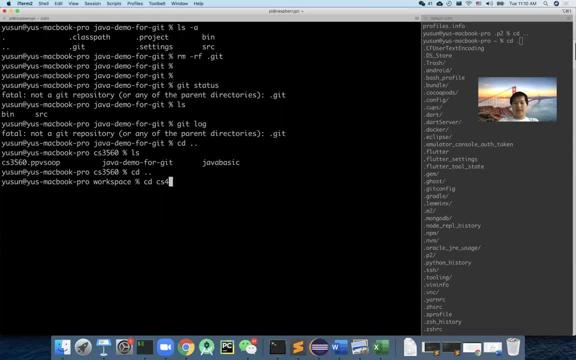 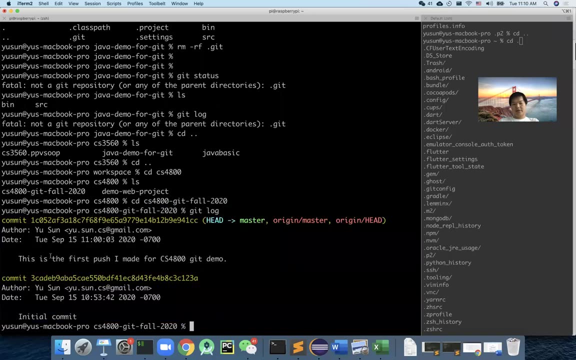 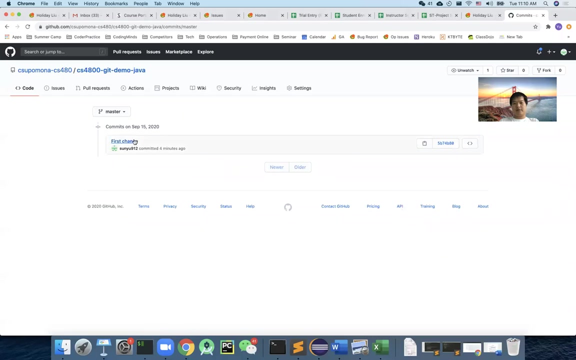 Oh, sorry, This is not a Git repository. Let me come back to the 480 class. I do Git log, All right, So you can see. it shows the list of commit I made recently with all the community messages And you can also see the same thing here in Git repository. 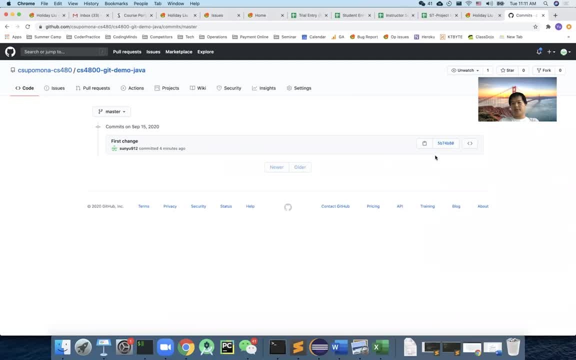 You can also see here that that's how we make a change and what a change you'll make, and then you can click on it. You can change, You can see. Oh, okay, So these are the things we just added to the repository. 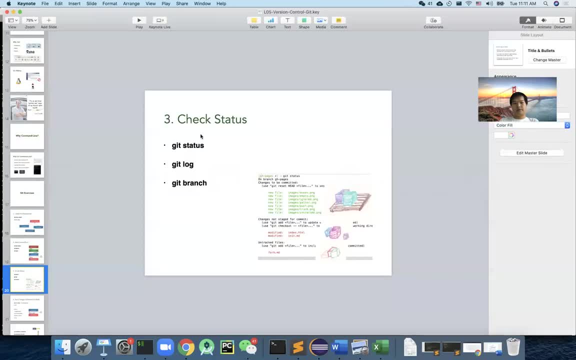 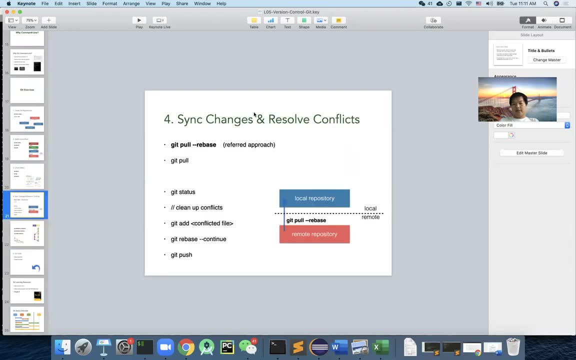 So very clear, All right. So these are the commands you need to know, All right. And finally, there is a kind of a synchronized command I need to show everyone so that you probably know it, Right? So here is one situation, the Bob Alice situation. 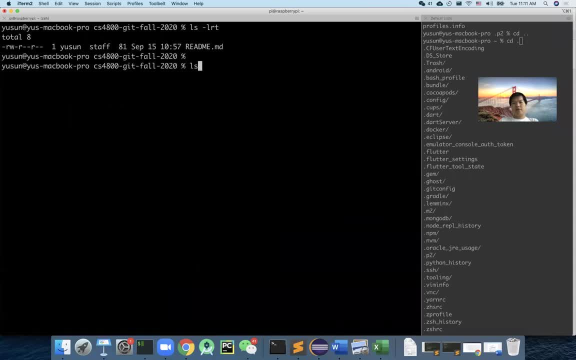 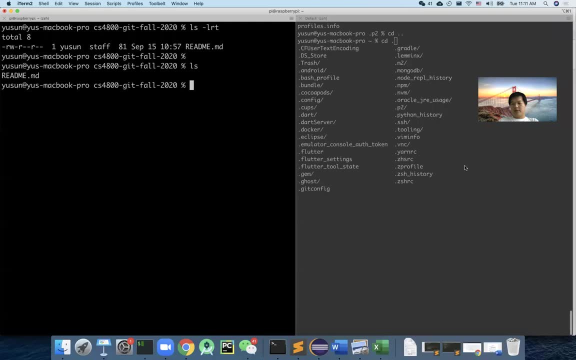 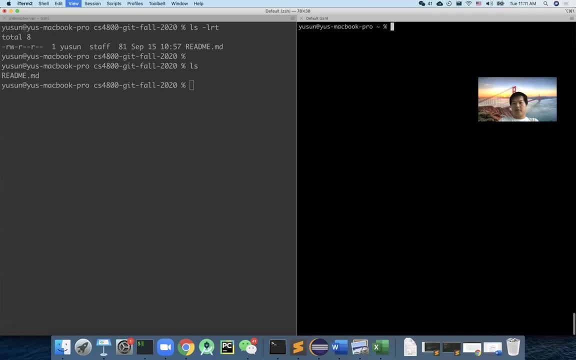 So let me come back to maybe again. I'll use a very simple example here. I'm going to open the two terminals here to show you, just so that you can assume. these are like. these are two different repositories. Okay, So I'm going to go to a temporary folder. 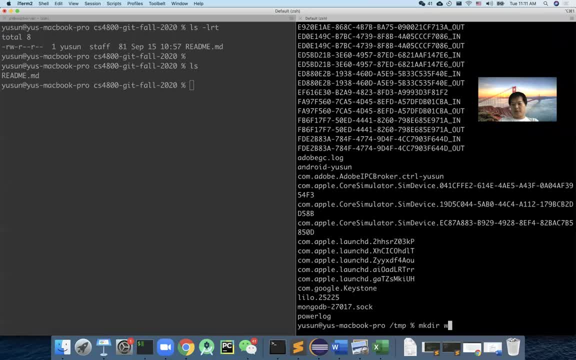 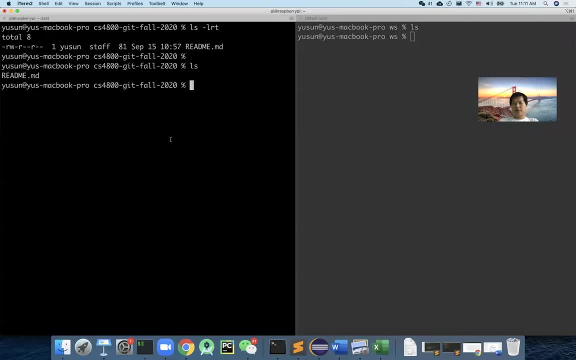 I'll go to a different folder here. Okay, I make repository workspace. All right, So these are the same computer. but assume these are two computers. Okay, Two different users. This one has a repository here, This one also has it here. 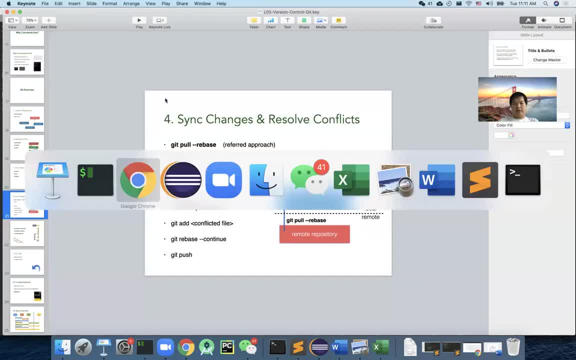 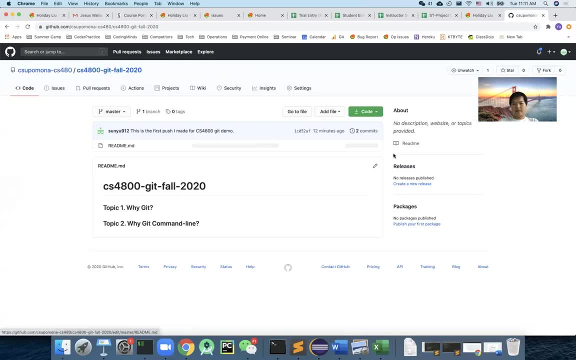 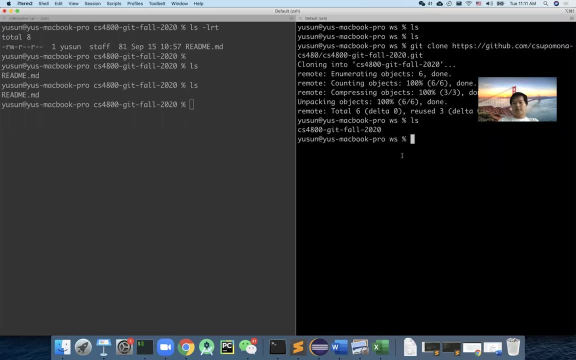 So I'm going to do a git clone, I'm going to clone this repository again, All right, So this one here and this one here, just like Bob Alex- example, they have the same copy. All right, This is the copy. 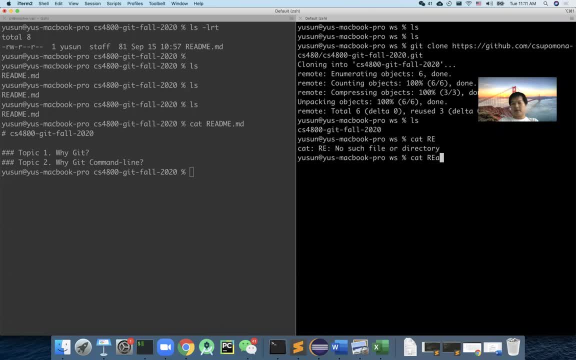 And this is copy. Okay, So this is the same copy. Okay, So these are the same copy folder here, So this is also another copy. All right, So they're exactly the same thing, but the two different user, All right. 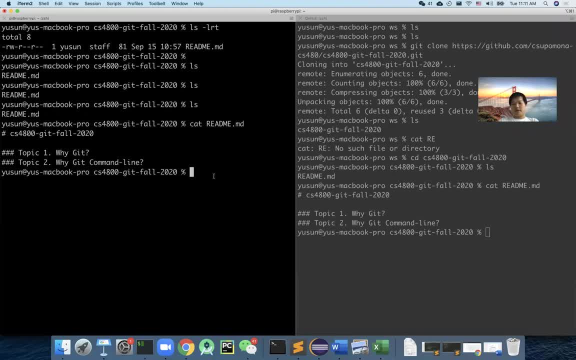 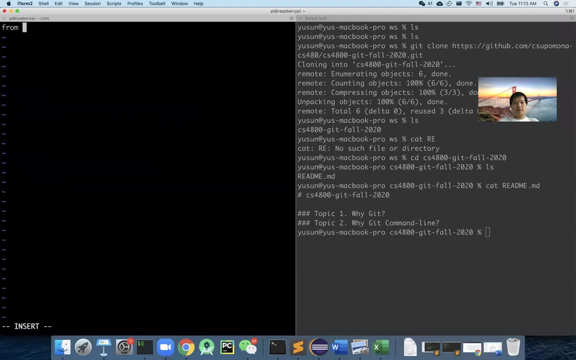 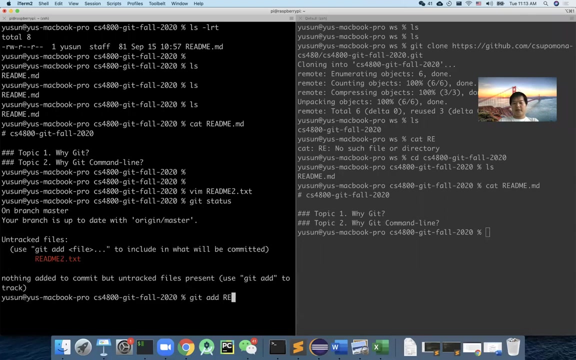 So we're going to push things one by one, Right? So, for example, I push something here called maybe I'll do another file. Okay, I'll do a, I'll do a readme2.txt. Okay, to txt from bob. look at status. so i'm going to do the add very quick, okay. 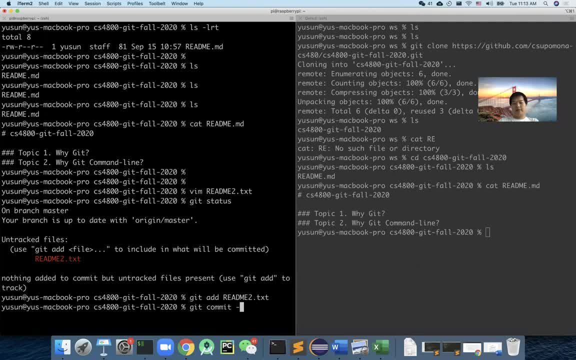 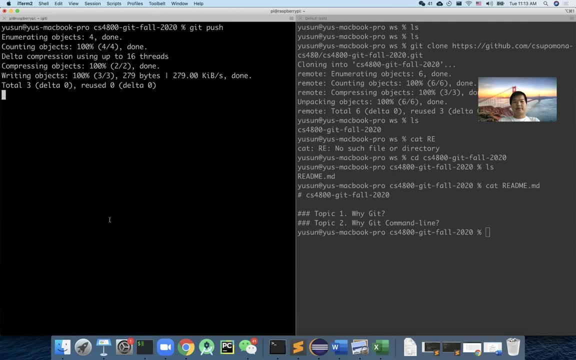 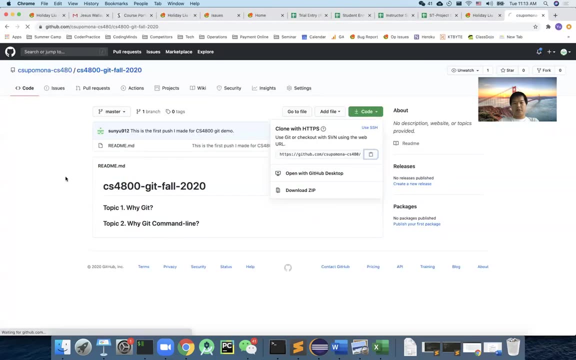 i'll just add this one here and do a commit message: bob's bob change, i can push. all right. so now this one here, push the new version and then you go to here, you refresh the repository. now there are two files, all right, but then this one here doesn't have that change, right, so this one still. 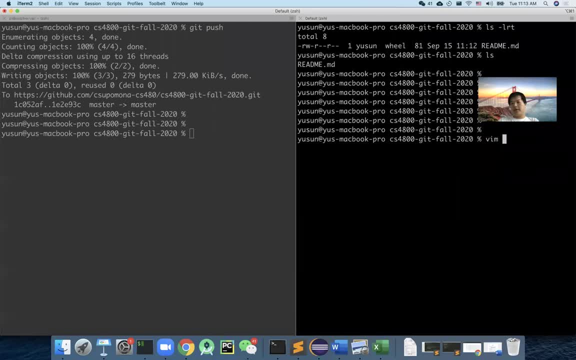 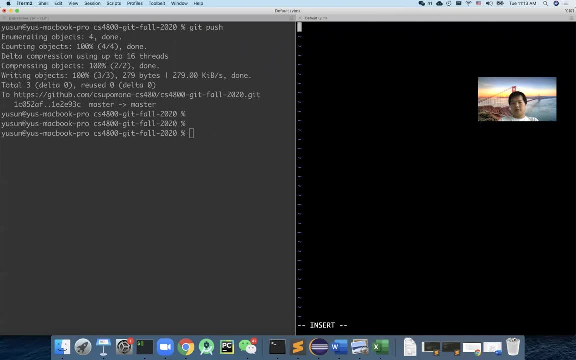 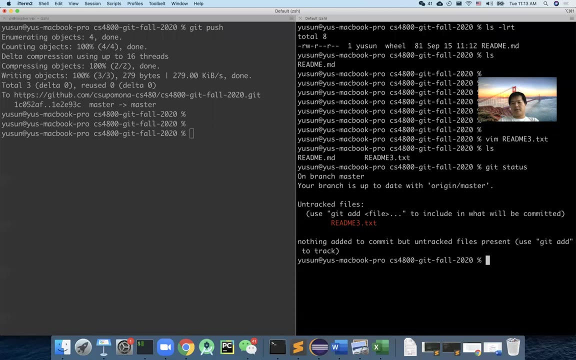 only has one file, but that's okay, i can also create my own. i will read me: uh, i'll do readme 3 txt from alice, all right, and then i just create another file to get add readme 3. i do get commit from alice, all right, so let's see this one. i'm going to do a git. 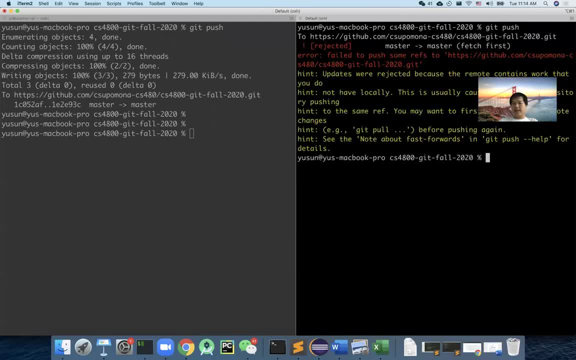 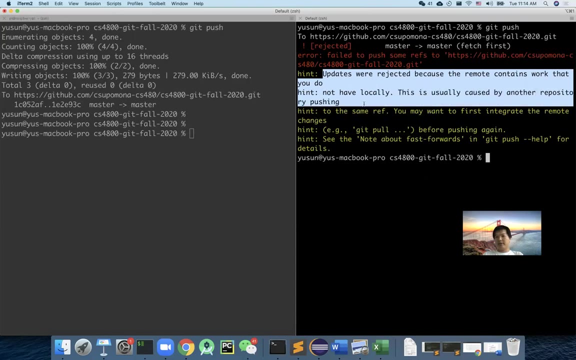 push, all right. so suddenly i saw this message. it said rejected, all right. and basically look at the message. they said that updates were rejected because remote contains work that you do not have locally. this is usually caused by another repository pushing to the same reference, so you want to. 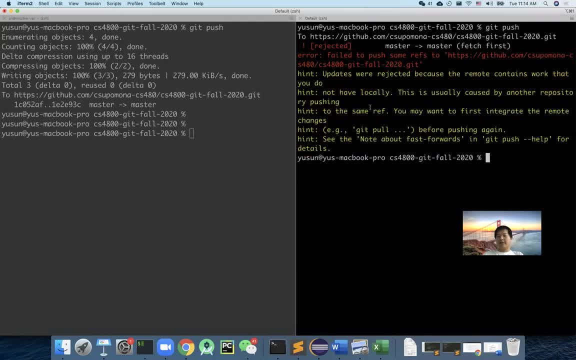 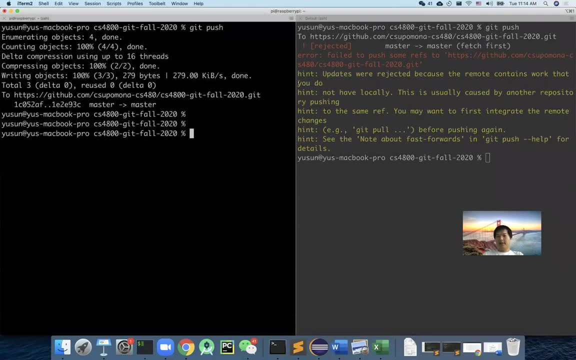 first integrate those and do all this command. so that's basically the scenario. we'll explain that your version is based on the older version because the bot just pushed something, all right. so all we need to do right now is to synchronize the change, all right, so i'm going to do a git. 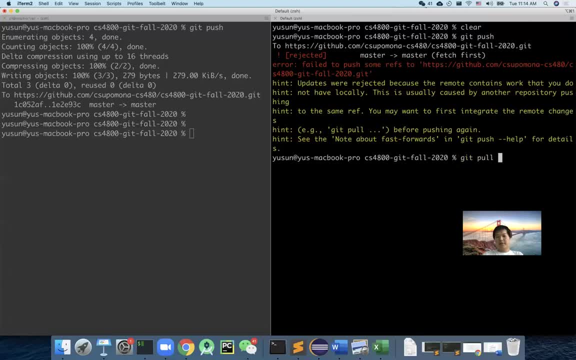 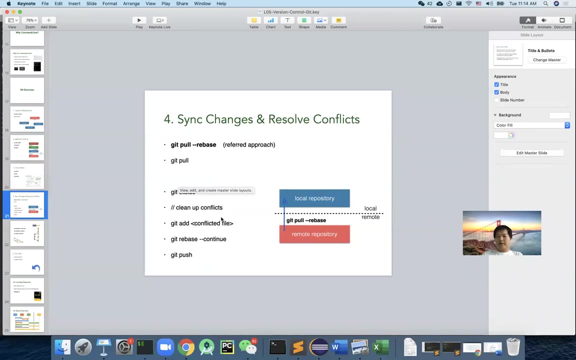 pull. that's the typical command. i also recommend you to get pulled dash, dash, rebase, all right. so i this is a highly recommended command. you can google the difference, but i'm just listing all this command i normally use right here to to uh re rebase your repository. so you're. 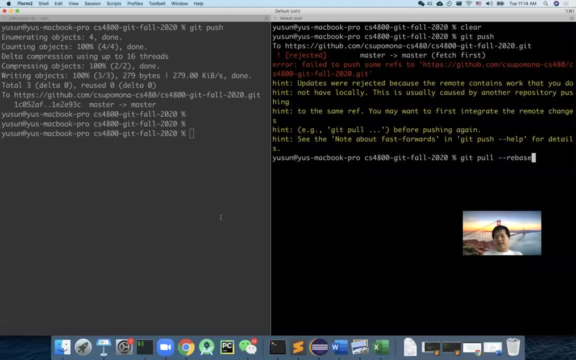 that you don't have to create the actual push to get. okay, you can look at the documentation, but it's it's very easy and very difficult to understand exactly what's going on, but i'm just telling you this is probably the preferred best practice for most of cases. all right, so that's. 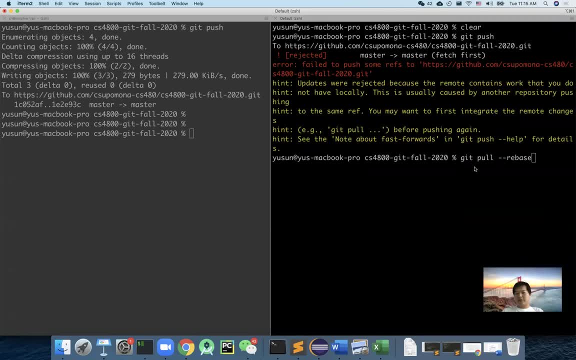 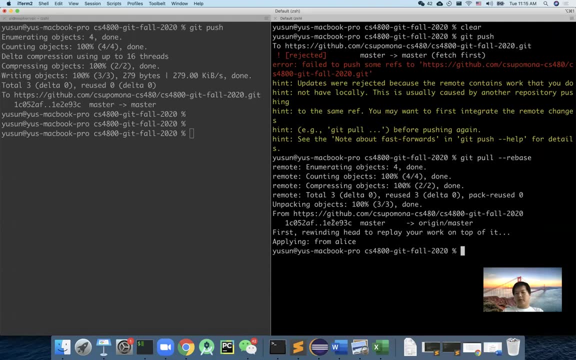 the one i normally use, but then let me run this one. you can see the results. so if you do this, all right, so it's actually automatically- update the change repository and try to merge the changes possible. and now, if i list the file, as you can see it has all these three. 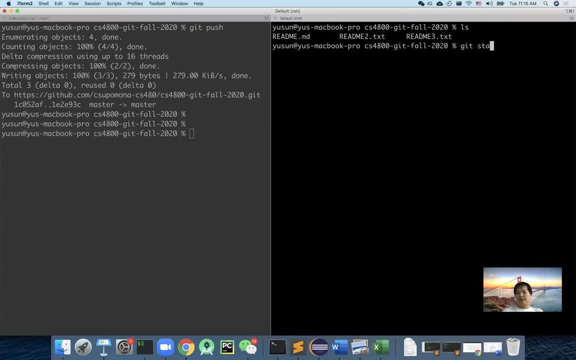 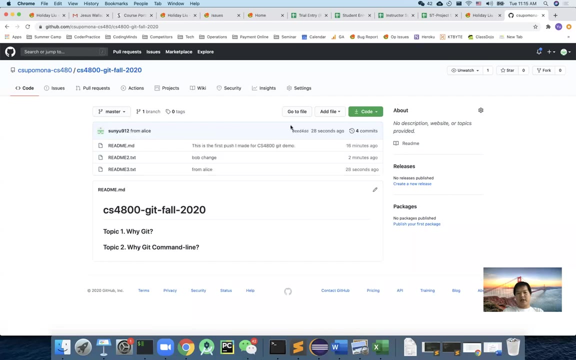 files. okay, one, two, three, all have it. and then if you do git status, and then you still have one committee, you haven't pushed this time. if i do git push and then you can push it, because now your version is synchronized, i go back to refresh and then we've got all the changes. 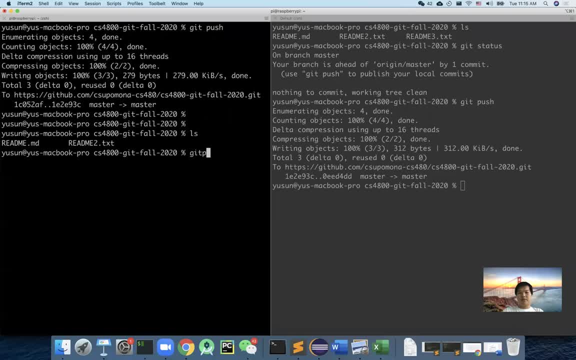 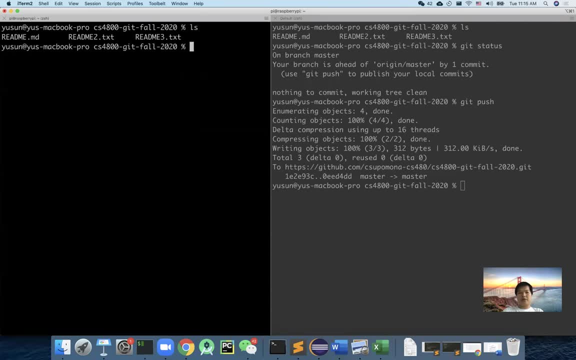 and if i come back here, this one only has two files. if i do git pull dash dash rebase, all right, so now it change, get all the changes. so now both versions have their own version has exactly the same changes. sorry, same same version, all right, so that's what you need to do. 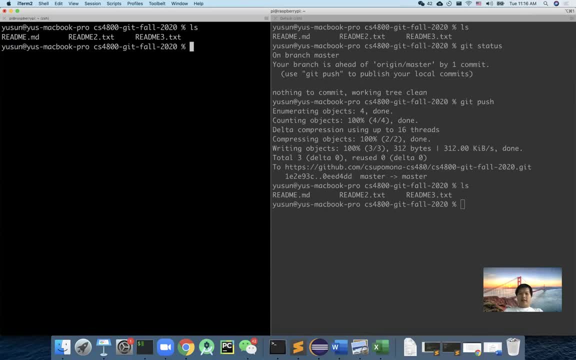 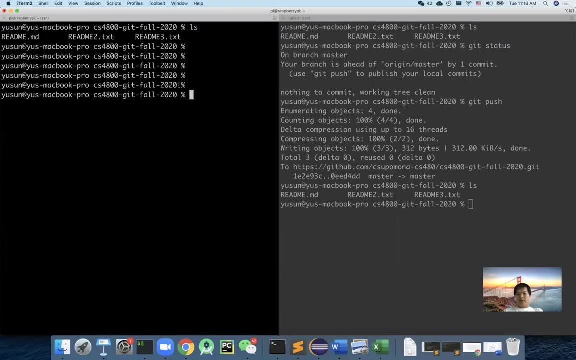 when you try to synchronize all the change. all right, but one more thing i i missed- i didn't talk, which i should- is i'll take you one more minute. all right. what if two people are are changing the same thing? okay, that's something you should be. 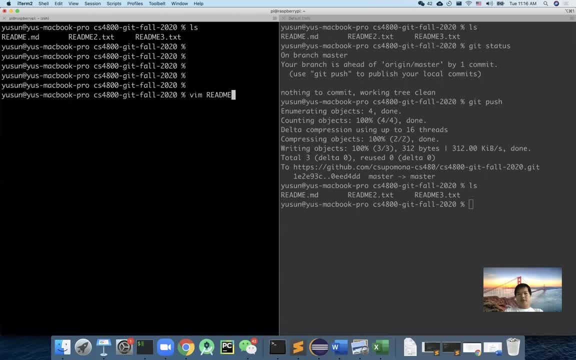 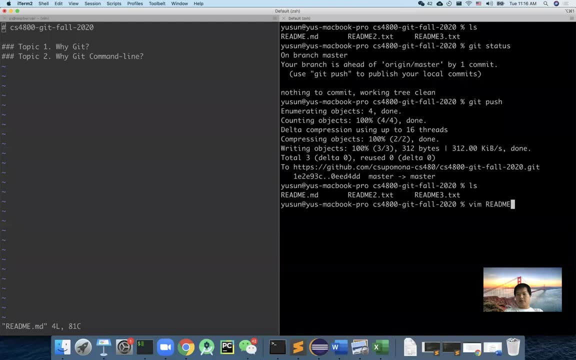 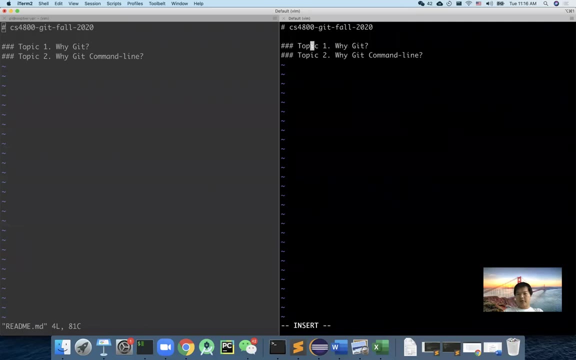 careful, all right, so if i'm bob, i'm changing this file here and then i'm alice, i also need to do the same. all right, so i might fix some. i'm adding like topic one. i'm going to change it to y get for version control, this one here. 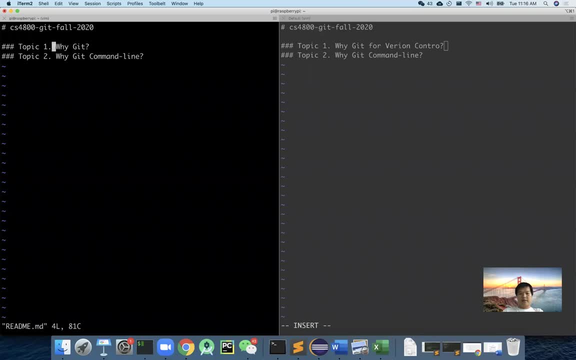 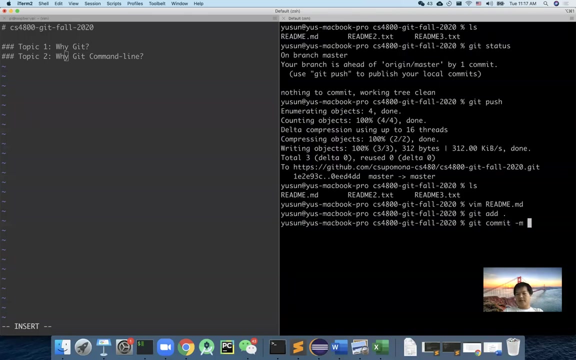 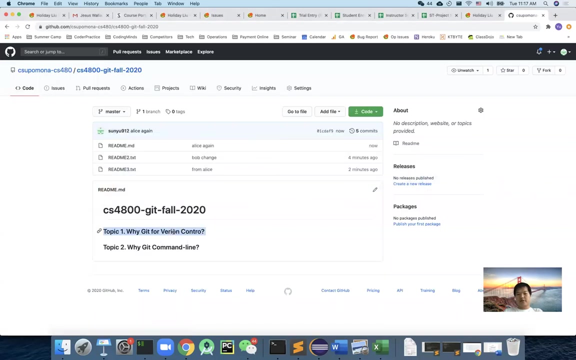 somehow i also feel this is something wrong. instead of saying topic one, say time, sort, topic column, all right. so alice finished hers. first, git, add, git, commit, get, push, all right, no problem, because i was pushing first. so you, you change this one first, all right, and then. 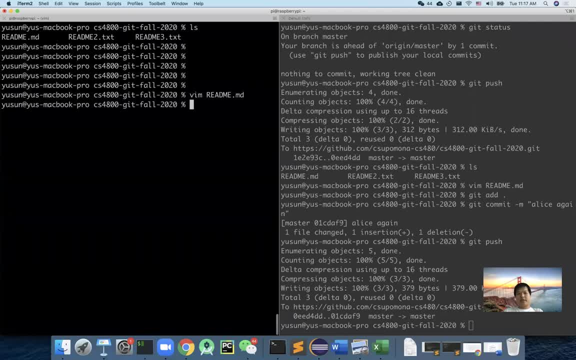 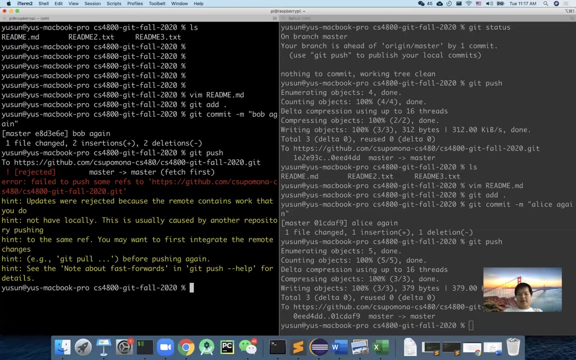 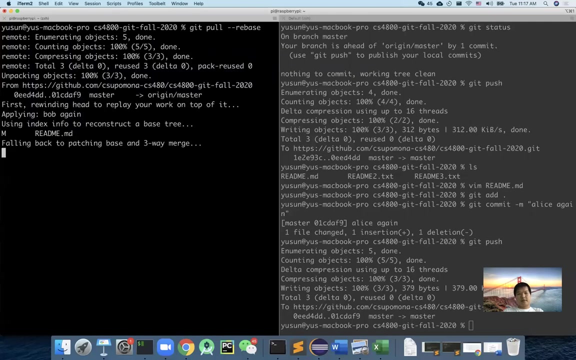 when bob finished his change, he saved the change. you do git add, git commit- all right. and then we do git push- all right, something going to change. you have to redo it, re-synchronize, and git pull dash, dash rebase, all right. and this time it says that. you know, i'm actually trying to. 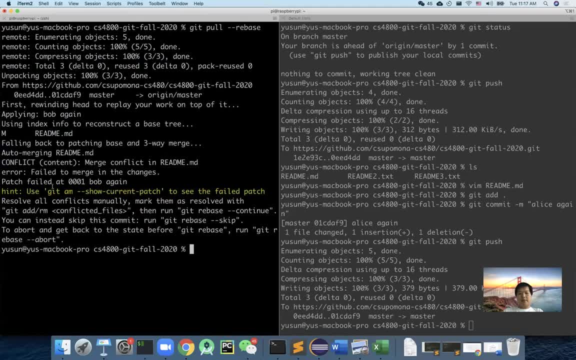 get updates and i'm trying to merge everything but eventually it said: fail to merge the change, all right, and then you have to manually resolve all the conflicts and marks and resolve all of those and then look at all the commands. so this time what happened is, even though you are trying to 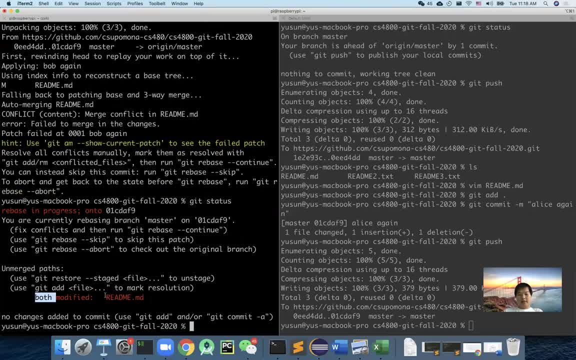 synchronize the code, but this time we found that these two developers make the same change, the same file, at the same position, so git doesn't know which one to pick. so that's why git has to leave that job for you to decide. So if I open this file here, readme, as you can see, the file has been changed like this: 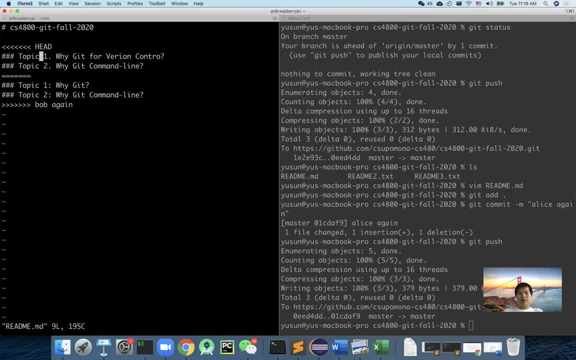 It says that you know, right now the head of repository in remote looks like this: That's exactly what Alice changed, And then this is a version that you have on your current local carpet. Which of this one do you want to use? 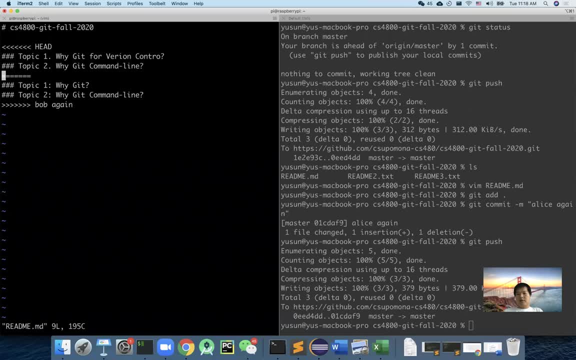 Again, because the git doesn't know who's right or who's wrong, And this one had to be done manually. So this is called resolving the conflicts, So I have to manually decide. oh, you know what? I think Alice's change makes sense. 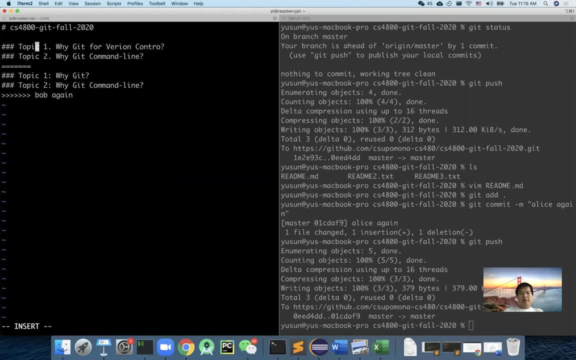 So I'm going to use hers, but at the same time I'm going to add my change on top of it And also there's a typo, so I need to fix that one And that's it. So the rest, I don't need it anymore. 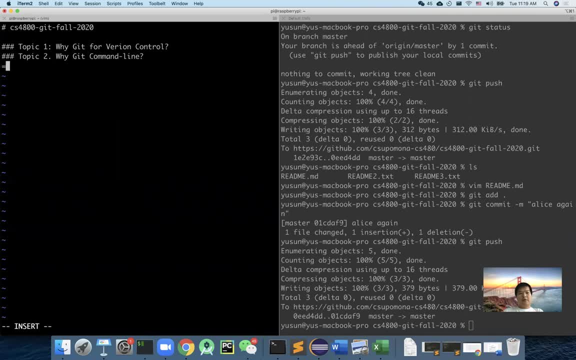 So I'll just delete it. This is called a manual: resolving the conflicts, Once you're done. Oh, by the way, I need to save also this one here. Once you're done, save the change, All right, Git status. 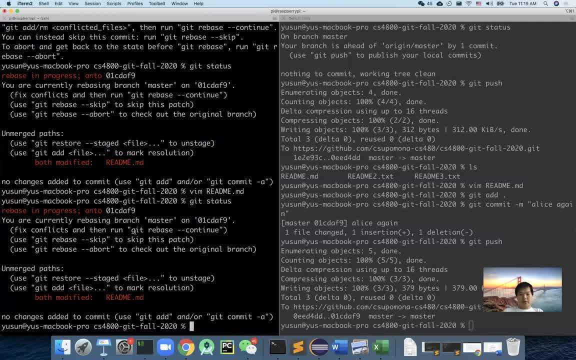 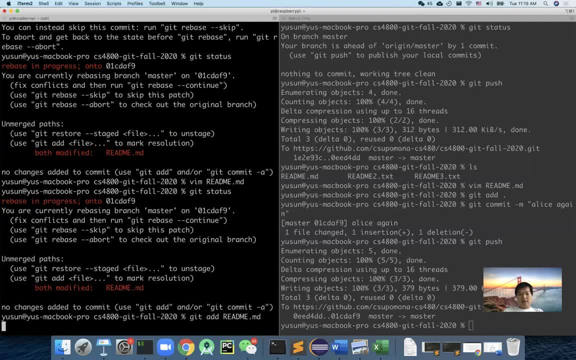 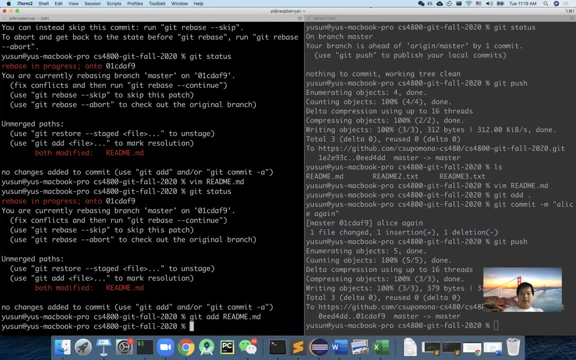 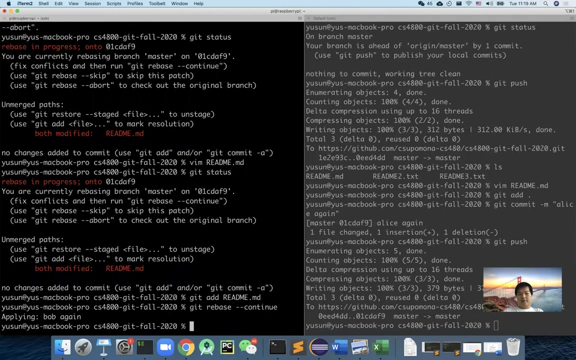 All right. So you need to follow this command here to finish this one. So git add: Why this one suddenly becomes so slow? All right, And then git rebase, dash dash continue, All right, And then we do git push And now you're finished resolving the conflicts. 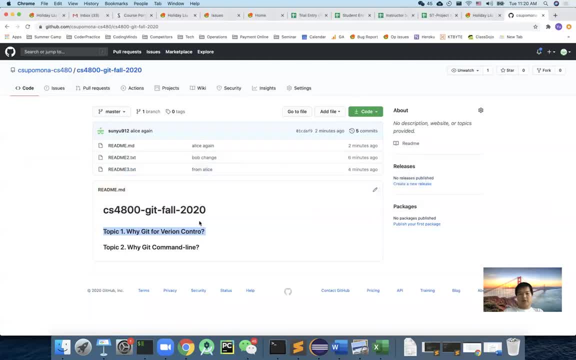 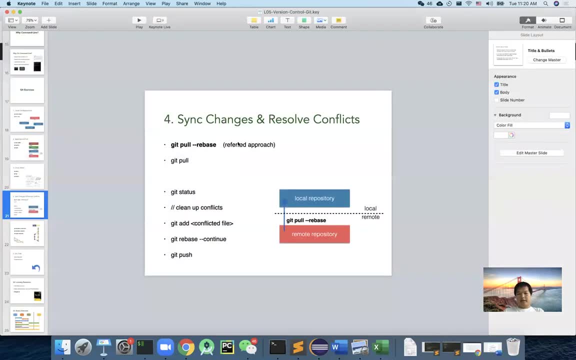 You push everything to the repository, So now I go back here. All right, So that's the latest version. Okay, So, because of the time, I don't have too many time to spend to talk about this one, but this part is one piece that you might face occasionally. 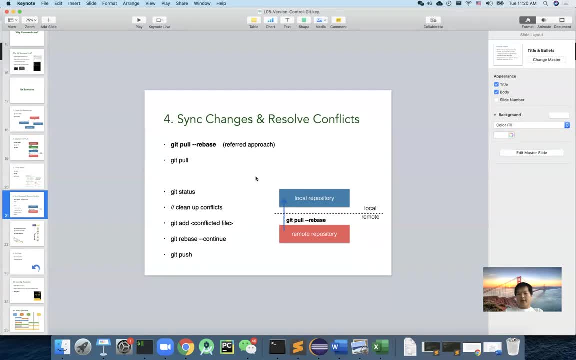 All right. So when multiple people are changing the same place of the same file, you will probably get the same result. All right, So that's the latest version. So now you can see that you will probably need to resolve the conflicts. Resolving the conflicts is nothing challenging.